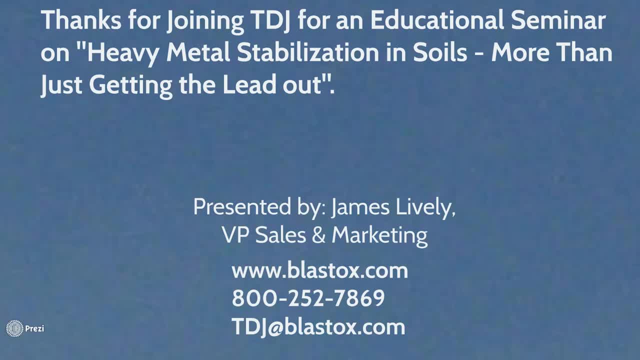 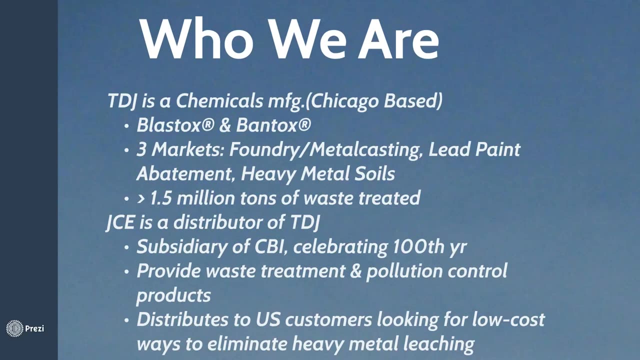 very garbled, so I have muted everybody else's mic on your end so that only my voice is being heard here. Without any further ado, let's go ahead and get into the presentation here. Before I just briefly describe our company, I do want to talk, kind of just set the table, We're not going. 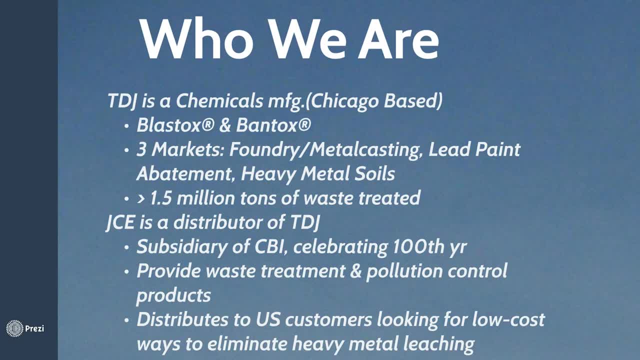 to go through the stoichiometry of every chemical reaction and what a chemical equation would look like. Rather, we've kind of just made it more of a layman's presentation here, where we're going to talk about lead and cadmium stabilization and how straightforward that. 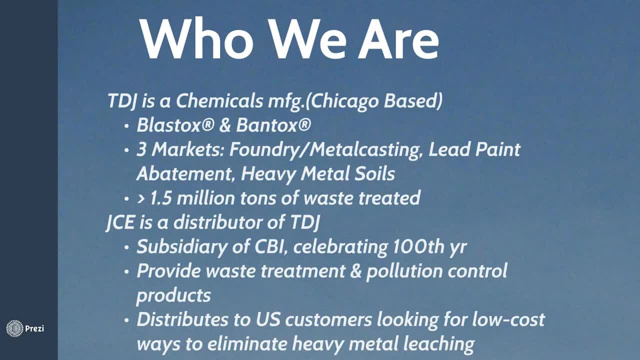 is, and then compare and contrast those two metals with arsenic, chromium and nitrogen. At the end of this talk we will also talk aboutMo selenium and compare and contrast the different types of stabilization methods, And then we will also discuss some different methods of mixing materials, whether it's our material or another material, and regardless of the types of heavy metals, the mixing method would be independent of that. And then, finally, we're going to end up with just a couple slides showing the relative cost of being able to stabilize a lead or cadmium. condition or coal, describing where it's put in and gather when youspeak one, in what way and to what extent. you should consider four. In addition to a lot of the other topics, we've got a list of batteries that could be used categorically in any kids' environment, including 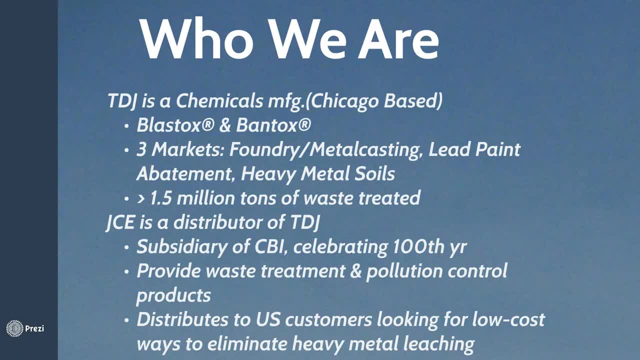 contaminated soil waste versus an arsenic, chromium or selenium contaminated waste. So, briefly, who we are. Again, my name is James Lively and I'm the VP of Sales and Marketing, And the TDJ Group is a firm that I represent. We are a chemical manufacturer located in the 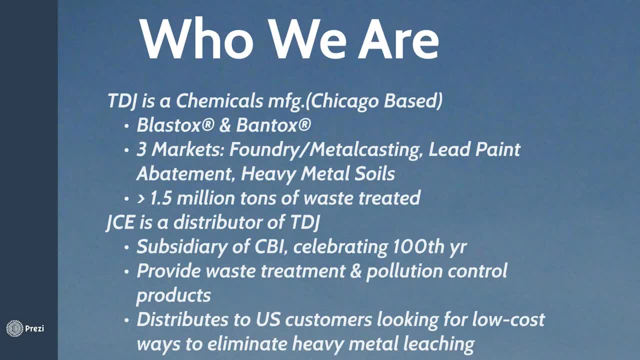 Chicagoland area. We've got a production facility about an hour and a half outside of Chicago. Our two primary product lines are Blastox and Bantox and we serve three primary industries that produce hazardous waste: The foundry industry that produces lots of casted metals. 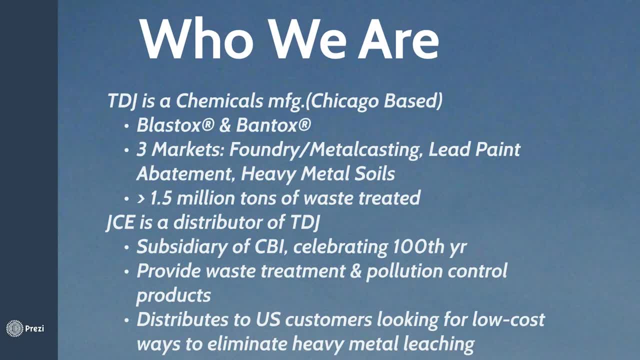 They produce a heavy metal contaminated backhouse dust that's collected off the furnace emissions that tends to be lead and cadmium concentrated. We also provide products to contractors that would be sandblasting lead Base paint off of bridges and water towers and other types of industrial structures. 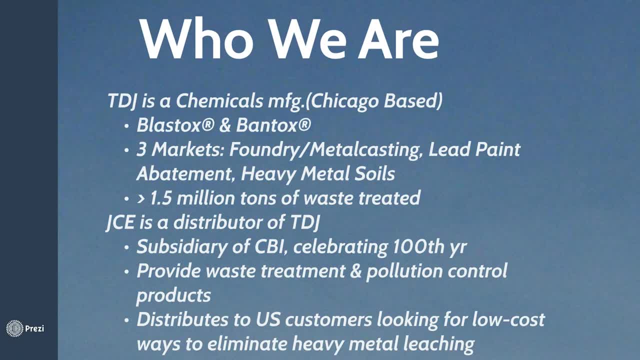 And, of course, today we're talking about soil remediation, which again is another industry that we provide our products to, And in the 20 plus years that I've been with TDJ, we've been able to successfully stabilize well over 1.5 million tons of waste. 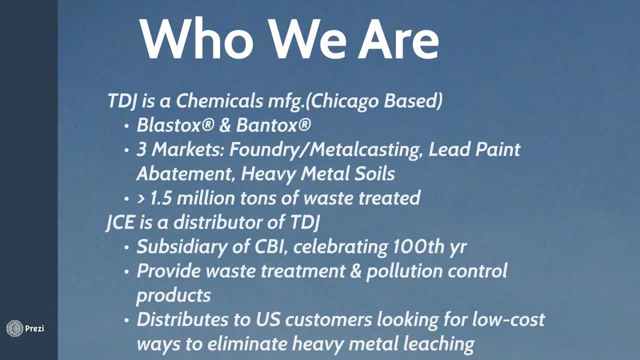 Our distributor here in the Midwest is J Carpenter Environmental, or JCE for short. They are a company that is a part of TDJ. They are a part of TDJ. They are a subsidiary of Carpenter Brothers Incorporated and Carpenter Brothers Incorporated. 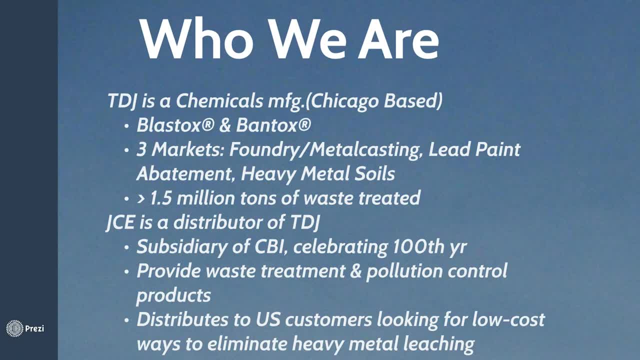 is celebrating their 100th year of existence this year, so clearly they're a very successful, long-term, stable company. They provide products to the foundry industry, but JCE is their environmental division that provides various types of waste treatment and pollution control products. 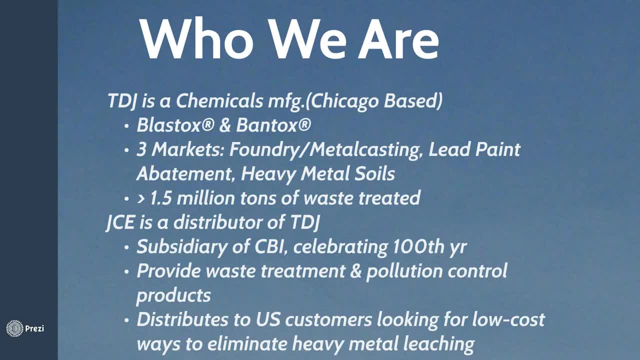 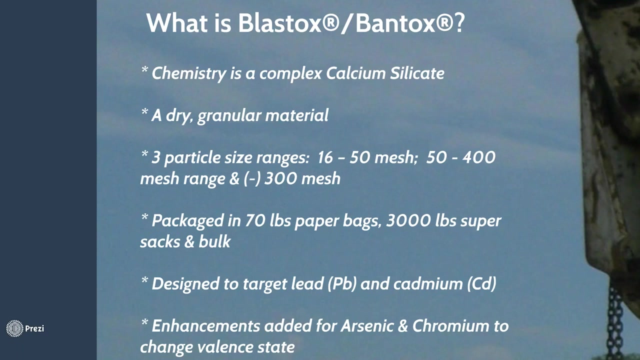 Overall the TDJ JCE team, are primary and our goal is to sell the material to not just US customers but really anyone in North America who's looking for a low-cost way to stabilize their heavy metal contaminated waste streams. So just very briefly, Blastox and Bantox, those are our two primary product names. 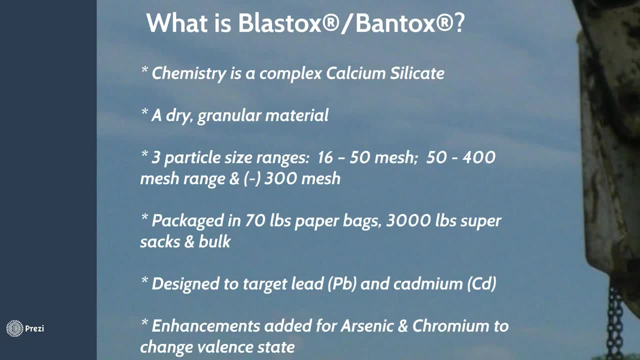 They are calcium silicates. They're dry granular material. We can provide them in a number of particle sizes. We can provide them in a number of size forms, depending upon what the application is keeping in mind. the smaller the particle size, the more reactive the surface area, so you get more bang for your buck typically when you go with a smaller particle product. 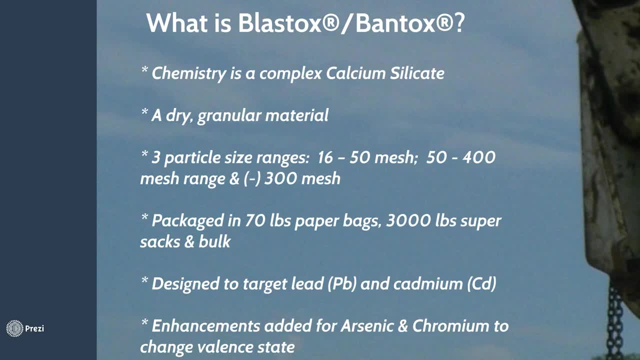 We provide them in standard packaging of 70-pound paper bags, 3,000-pound super sacks and bulk capacities as well, and we'll talk a little bit more about the super sacks, because they lend themselves to easy application on a job site. 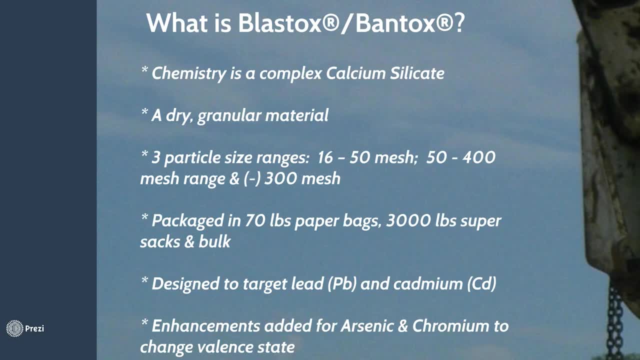 This calcium silicate is designed specifically to target lead and cadmium, which we're going to talk about here briefly, but then we can also add additional enhancements or other reagents that would reduce or change the valence state of arsenic, chromium and selenium. that would make them more conducive for silicate stabilization. 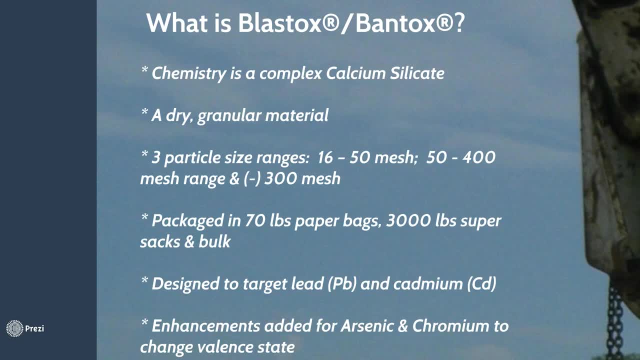 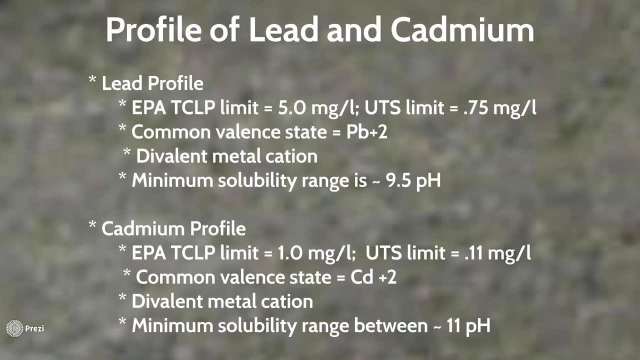 What I want to do is just kind of give everyone a little bit of an understanding of the different types of silicate that are available, Some of the characteristics associated with lead and cadmium. I want you to keep that in mind because as we get to the other three more unique difficult metals to stabilize, this information will be good to compare and contrast. 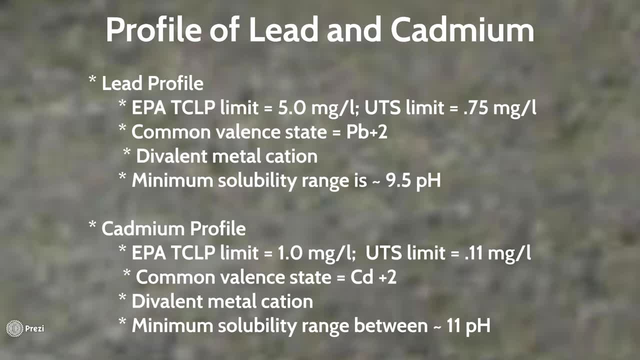 The TCOP limit for lead. I would guess most people on the line probably know that with the TCOP test it's five milligrams per liter, not milligrams per kilogram. Milligrams per kilogram is a total. If you look at how much lead there, this is how much is leachable. 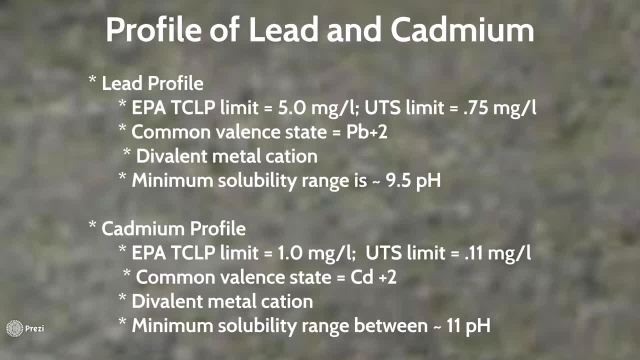 The UTS standard, or universal treatment standard, for lead is 0.75, and I should say that universal treatment standards in general- not always, but in general- tend to be lower than TCOP values, because it's the EPA's way of saying: once you have hazardous waste, a hazardous soil, then you have to treat down to below not TCOP value but universal treatment standard. 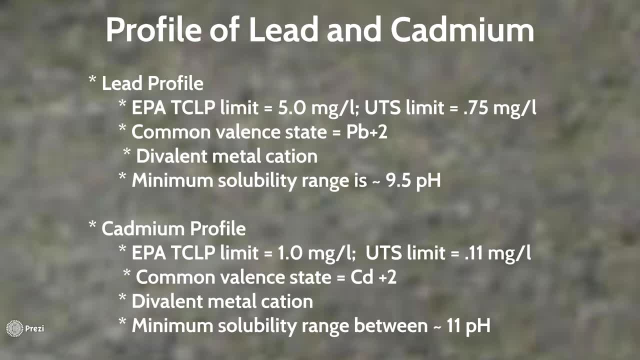 Okay, Thank you, Thank you. Thank you, Dr Haley. All right, So, as I said, I'm going to just make sure I'm doing this correctly. I am not going to be using the same standards, so that target for that objective could change for your project. 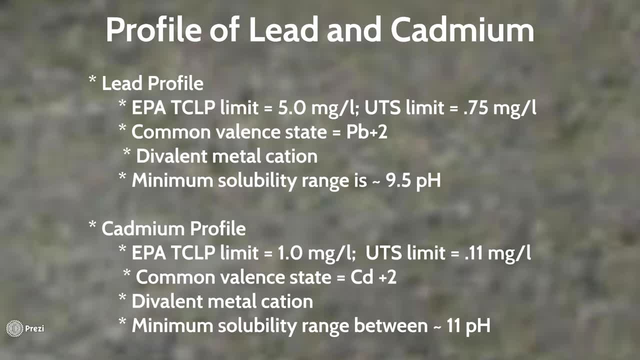 So clearly. you want to know upfront is what my bright line to pass. is it five milligrams per liter or is it 0.75 milligrams per liter? Lead and cadmium are both plus two divalent metal cations, meaning that their valent state is plus two. 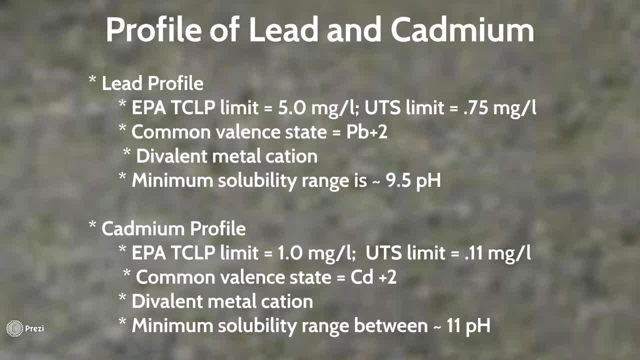 And that'll be important, as calcium and potassium are in the same state. That's why they're called valent states, because they're not divalent calcium silicate. if you understand that chemistry, calcium is an, an alkali earth metal that also is a divalent metal cation, so upon reaction you would have a. 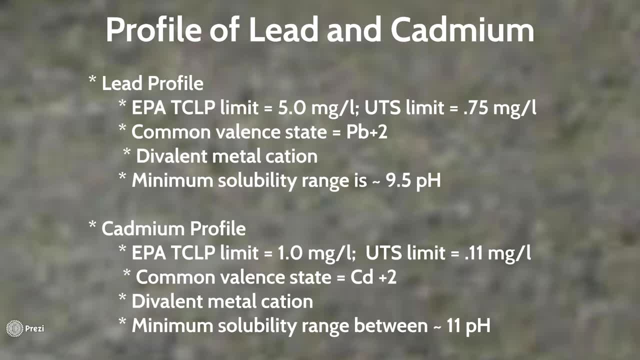 substitution reaction of the lead or the cadmium, replacing the calcium for an insoluble heavy metal silicate with lead, and we'll see that graphically in just a moment. the minimum solubility range is about nine point five. for cadmium, the TCLP limit is lower, at one milligram per liter, and, of course, a UTS value is even. 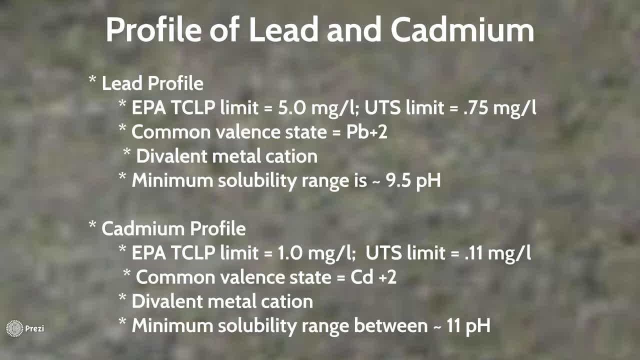 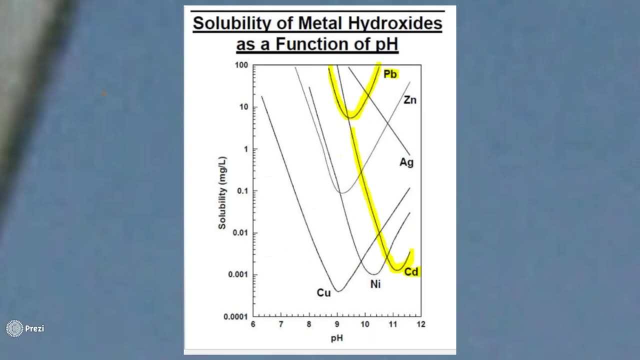 more stringent at 0.11 milligram per liter. its common valence state, as I mentioned earlier, is also a plus two divalent metal cation. its minimum solubility range is about 11. and the reason that's important- I've kind of illustrated that graphically here. 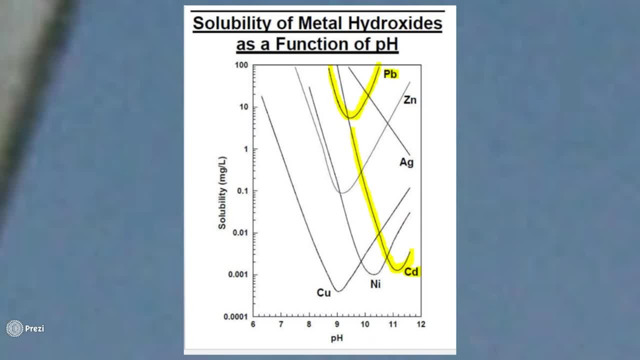 where I've highlighted toward the upper part of the graph, you'll see a horseshoe shaped curve with a lead highlighted. if you were to take a pen and draw at the bottom of that curve straight down, you'll see that that minimum solubility range is about nine and a half standard pH units. if you slide up the pH scale to 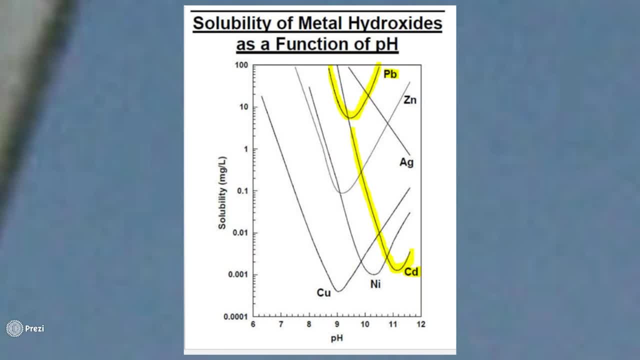 about 11- 11.5, you'll see that you've reached the minimum solubility range for cadmium. in other words, if you can modify the chemistry or the chemical environment to have the pH value elevated, you can suppress the solubility of lead and. 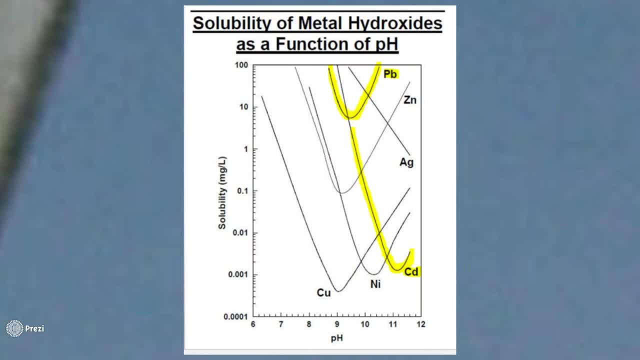 cadmium, by then precipitating out as hydroxides and not being soluble by pH adjustment alone. now I would caution people against using that, because pH is a temporary adjustment that would not create a long-term stable waste. in my opinion, that could cause some issues down the road in terms of those. 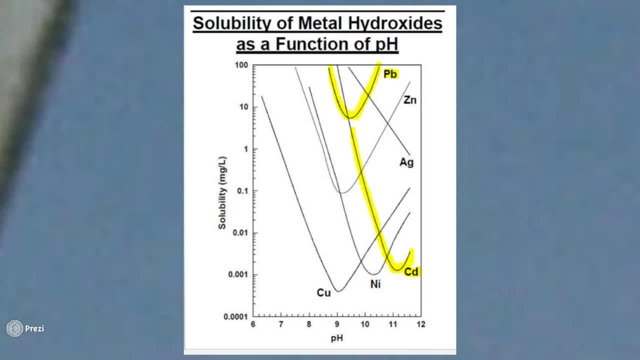 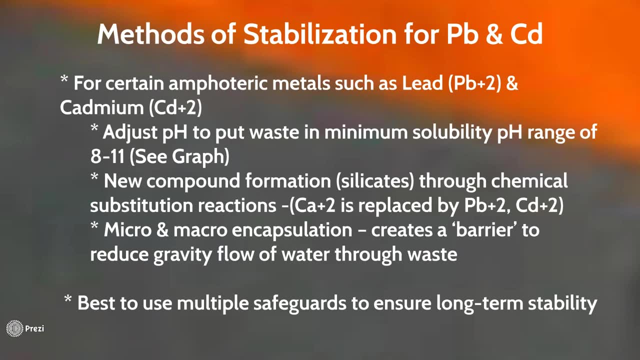 materials being available for leaching again once the buffering capacity has been eliminated. here's a list of the types of stabilization approaches you can use for lead and cadmium, but I would strongly urge you to consider using multiple of these again as a way to ensure long-term stability, as I 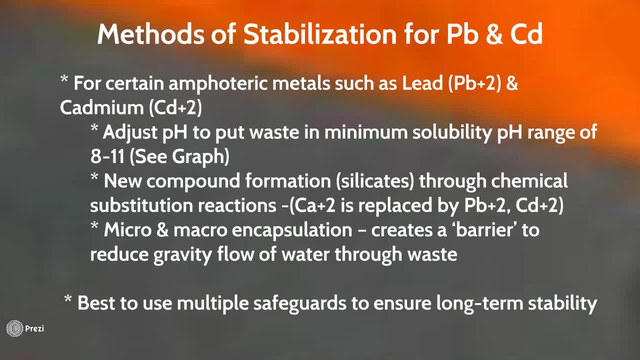 mentioned earlier. you can see that that minimum solubility range was between eight and a half and 11 for lead and cadmium. so you can add a calcium oxide or magnesium oxide as an example to artificially increase that the pH value and you're going to not get lead or cadmium to leach out. 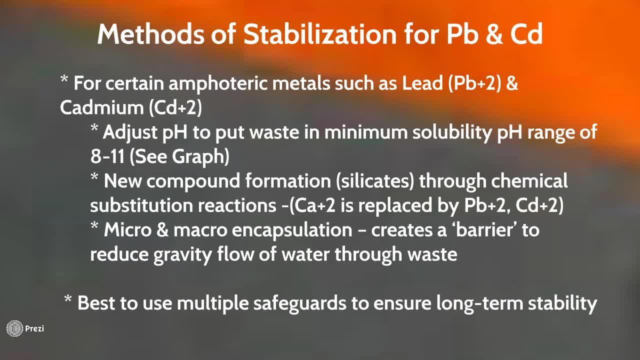 but the problem with that is calcium oxide and magnesium oxide don't form a long-term stable compound the way a silicate, perhaps, and other reagents would. so again, I would caution you against just using those materials as a way to achieve TCLP or UTS compliance, as I alluded to earlier. calcium in the 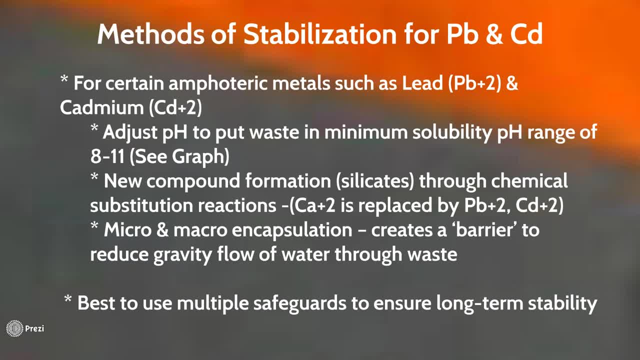 calcium silicate matrix is a plus two ionic form. you'll remember that lead and cadmium was as well. so when the calcium disassociates and leaches off of the silicate matrix, there's now a cation void site where the lead and the cadmium have an affinity to attach to. so 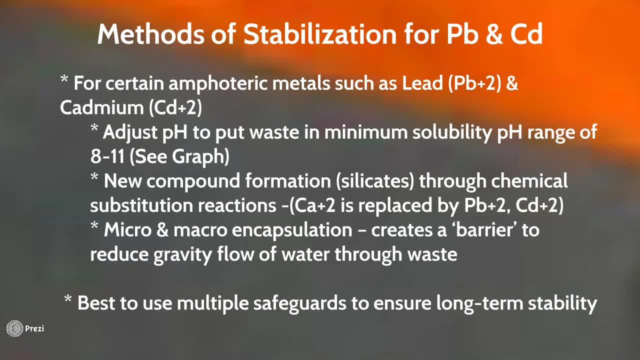 that is a chemical reaction, as is a pH adjustment. the third reaction really is a physical reaction, where the- you know the fancy terminology that we we like to use- we call micro and macro encapsulation. in layman's terms, that means that it solidifies or helps to create a physical barrier around 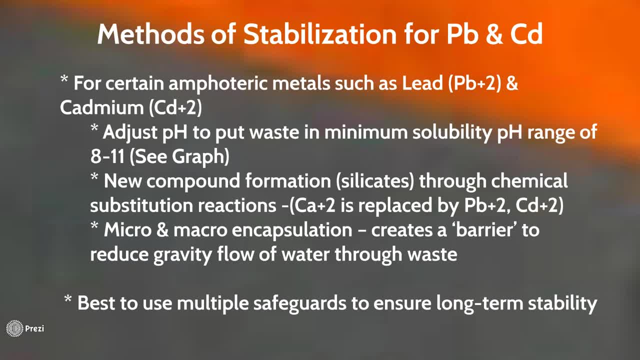 individual particles as well. as you can imagine this entire: a roll-off box being dumped into a landfill and, upon exposure to moisture, forming a crust around the outside, as well as having the materials inside to harden up, where you would have pH adjustment and chemical conversion, as well as encapsulation, all working together. 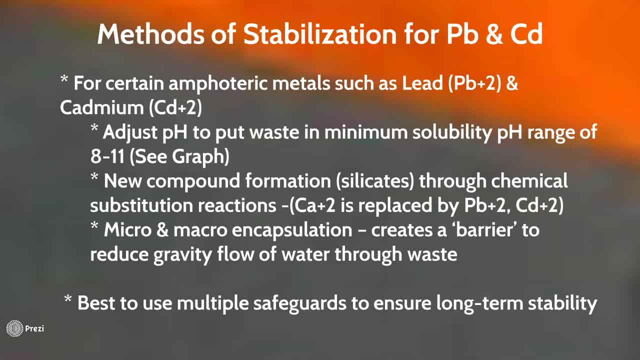 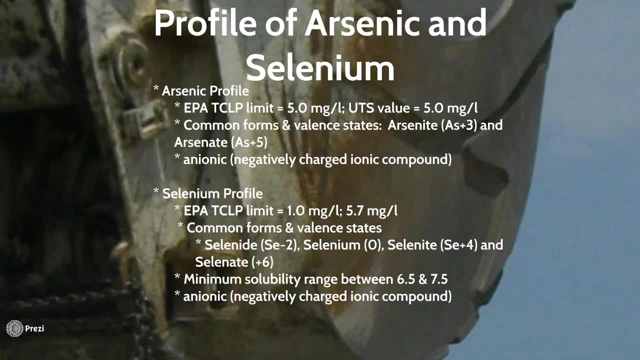 ideally as a way to create long-term, stable heavy metal waste. keep in mind what we had mentioned about the profile of cadmium and lead. those are both single valence charges at plus two. when we get into arsenic, selenium especially, but also chromium, you'll see that there are multiple valence states. 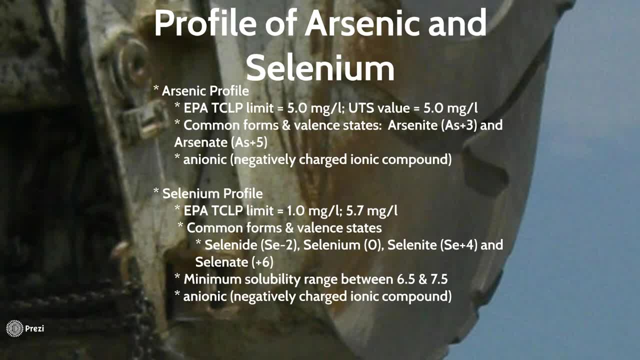 with arsenic. it's important to know that the tclp value is five milligrams per liter. interestingly enough, the UTS value is also five milligrams per liter, and the reason that value is not lower is because EPS set the value at a comparable rate and that tends to suggest the difficulty in being able to. 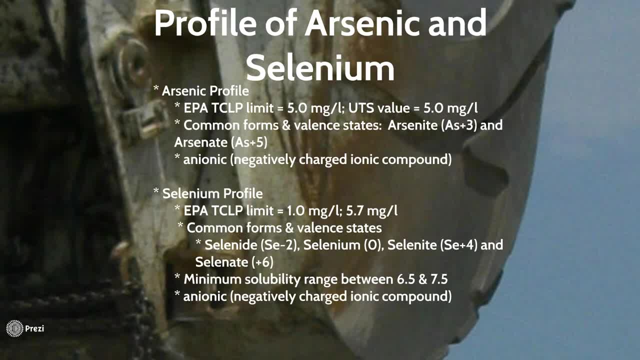 suppress or stabilize arsenic so that is no longer soluble. of the two common valence states are plus three or arsenite, and plus five is arsenate, and when they're in combination with other compounds they form an anionic compound. just a quick backup on anionic versus cationic, if you remember back in high. 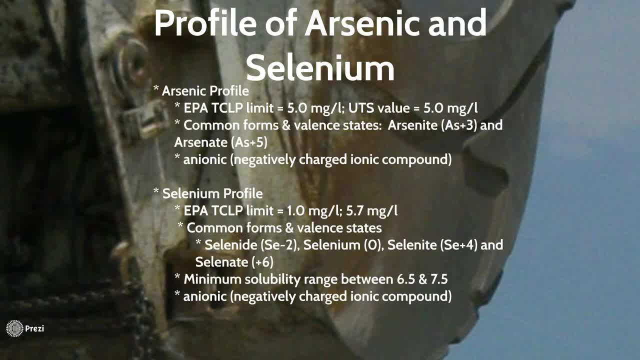 school chemistry, cations are positive, anions are negative. when these materials- arsenic that is- form compounds, they tend to be negatively related to the carbon, so they tend to be negatively charged compounds. that don't lend itself necessarily to either pH adjustment or or chemical conversion, in relying just 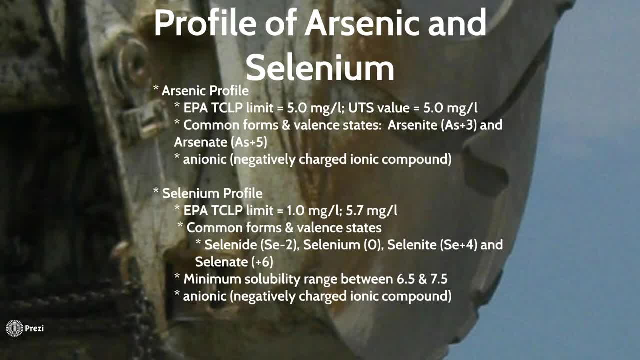 upon a silicate or other compound reaction. for selenium, the tclp value is one and, interestingly enough, the UTS value is five point seven, again speaking to the difficulty of being able to achieve compliance. so in theory it's a waste, exceeds one point zero and you add something to it as long as it's under. 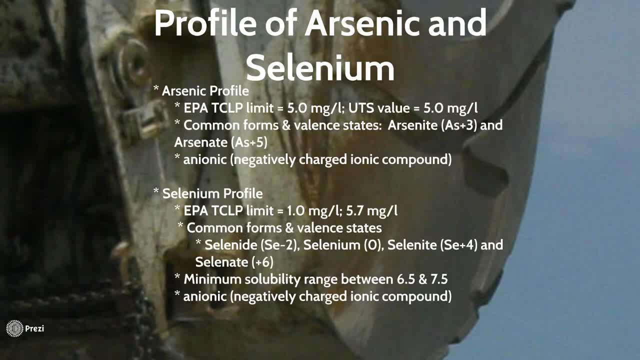 five point seven. you've achieved that treatment, but the the real intent and spirit of the rule isn't to try to play games between the tclp and the UTS, but it's to add something that will keep the solubility of selenium under five point. 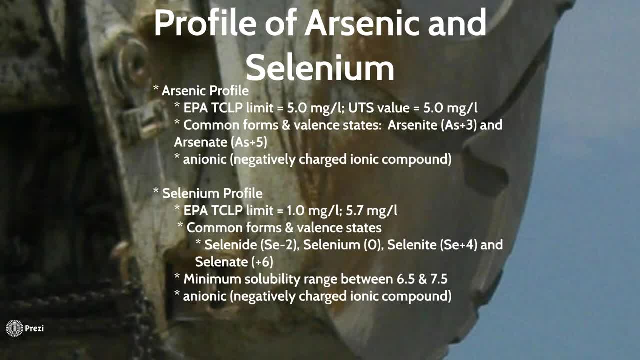 seven milligrams per liter. again, multiple valence states. selenium of the three is the one that has the most types of valence states, both a negative charged particles at minus two, which is called selenide selenium with a zero valence charge just simply means it's metallic. so if it's lead or cadmium and 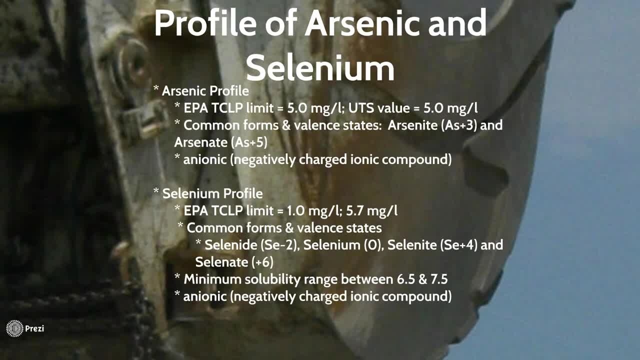 you see the charge at zero. that simply means it's the metallic form of that heavy metal. then there's selenite, which is a plus four valence charge, and then selenate, which is a plus six charge. now, their selenium does tend in some forms to have a minimum solubility range between six and a half and seven. 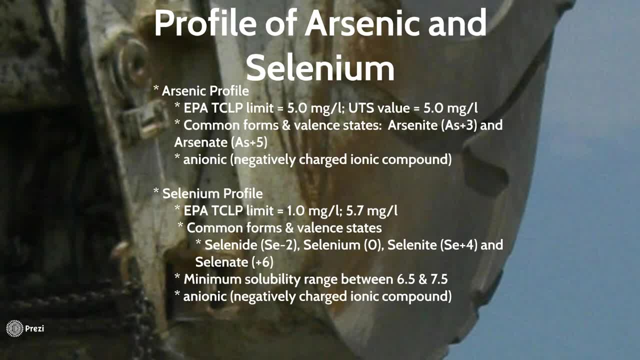 but if you remember cadmium and lead, they were eight and a half and higher. so if you try to hit the minimum solubility range of selenium and you also had cadmium, it would be nearly impossible to hit both minimum pH ranges as a way to 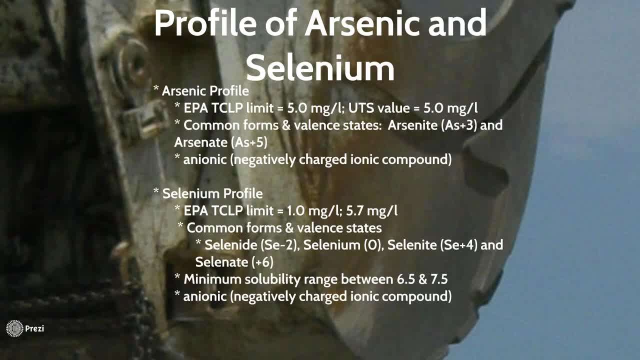 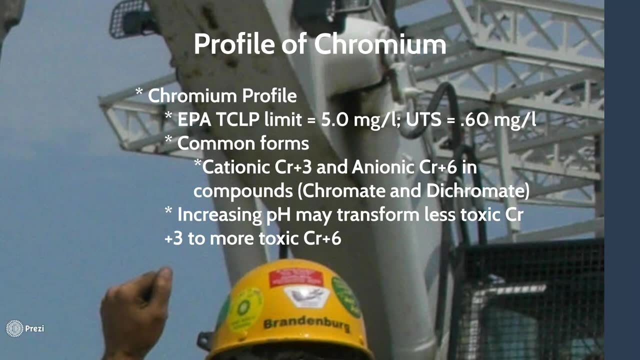 control the solubility by adding a pH buffering material only. and again, selenium. it is an anionic compound that it forms with with other materials. and continuing on the multivalent state heavy metals, let's discuss chromium, where the chromium TCO p limit is five milligrams per liter and the UTS value. 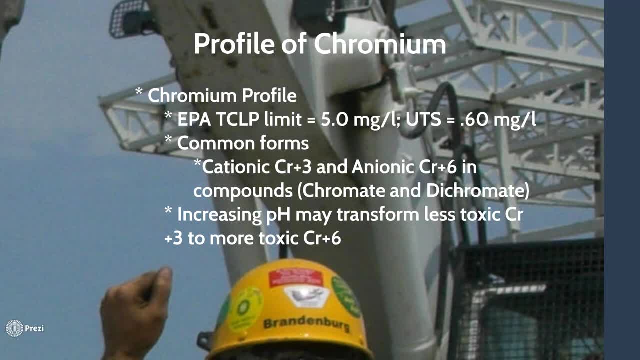 is point six milligrams per liter. it's lower and more stringent than the TCO p, kind of following the traditional EP approach where the UTS value is lower than the TCO p value. chromium has two different forms that tends to be present in. they're both positive valences at 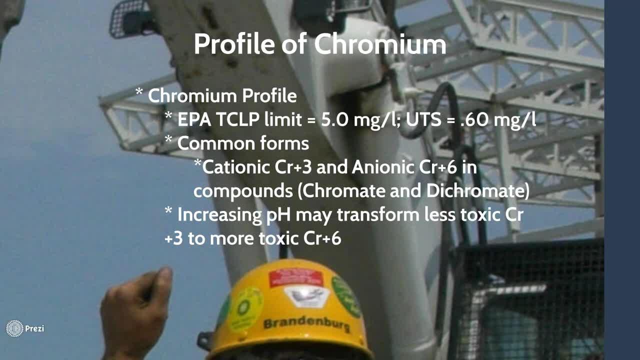 plus three or plus six, where you'll hear the terms trivalent and hexavalent- again just speaking to the number on that charge- and with the hexavalent they tend to be either chromates or dichromates when you look at the chemical form. interestingly enough, if you increase the pH and you've got a, 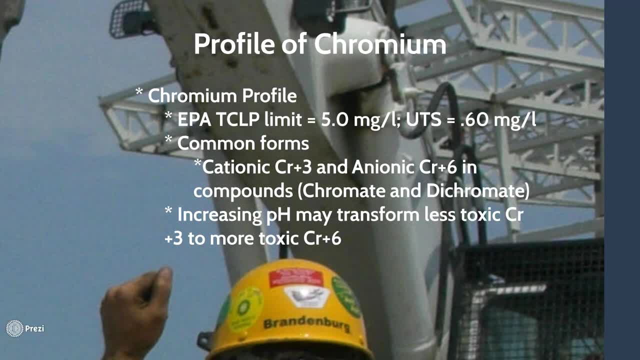 chromium waste because of the the potential for oxidization there you could actually increase the valence charge from plus three to plus six, and plus six is more mobile and more toxic than plus three. so if you had chromium and cadmium and you relying upon a pH adjusting material only, you could 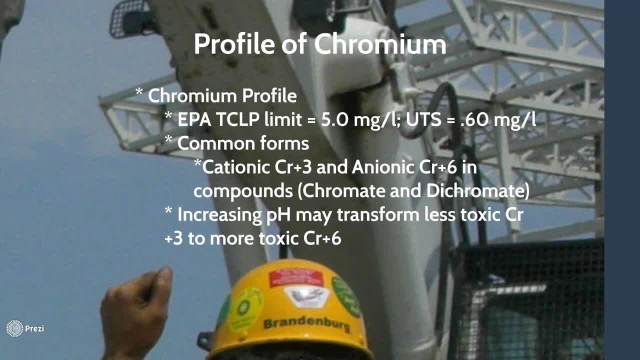 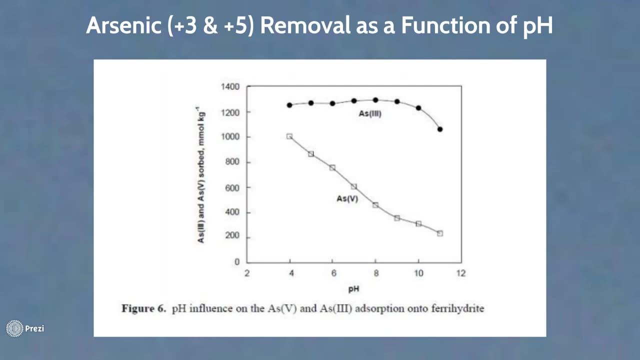 stabilize the cadmium or the lead, but by raising the pH you could actually cause the chromium to become more soluble, thereby causing a problem while you're trying to eliminate one. I've got. the next three slides are a series of of graphs that basically speak to how the solubility or the absorption rate of these materials to other 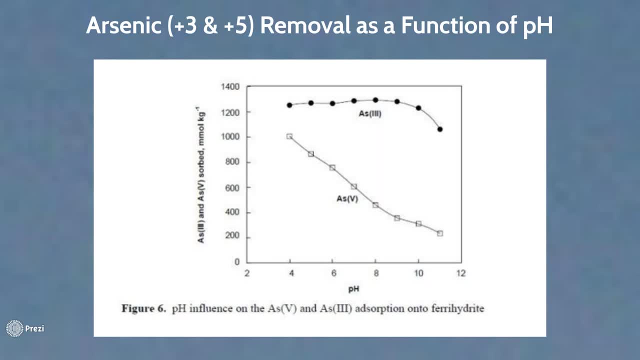 materials that would lock them up are being influenced by pH. so this is for arsenic and you can see where it's got both the Roman numeral three and the Roman numeral five. the line across the top is Roman numeral three, four plus three and the ones going more in the diagonal is a plus five valence charge. 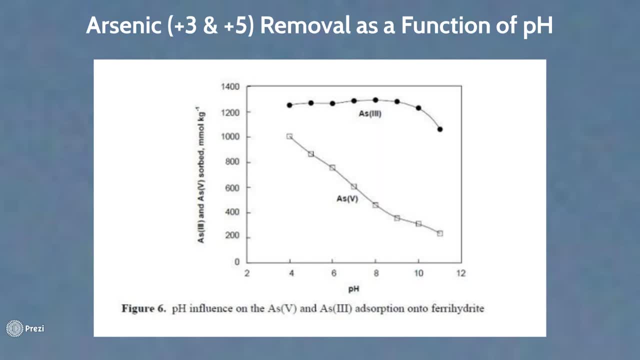 pH is on the x-axis. the y-axis, going from bottom to top, shows an increasing ability for these materials to be sorbed on to another product or on to another compound. in this case you can see it's ferrahydrite. so if you look at a s five, 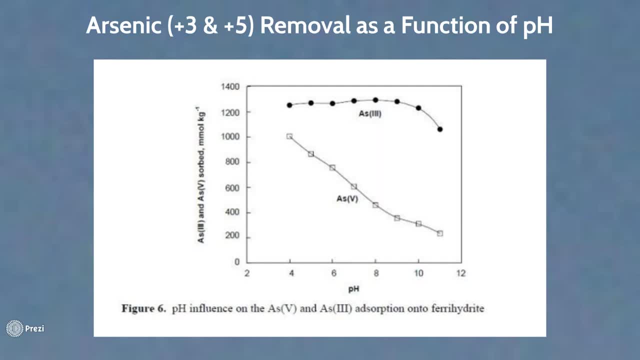 or plus five. as you increase pH, the ability for this material to be sorbed goes down. in other words, you increase the pH, the solubility goes up. now it's pretty stable for a s three, where you can see that up until over a pH of 10 it doesn't. 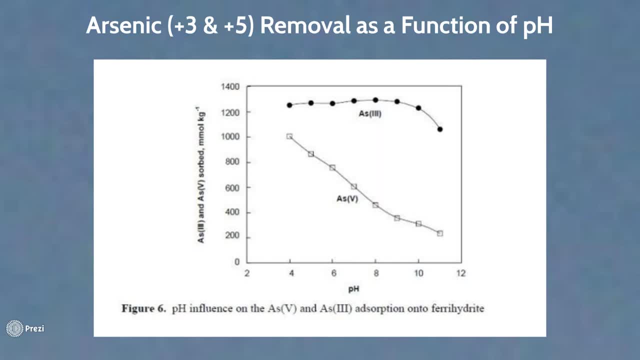 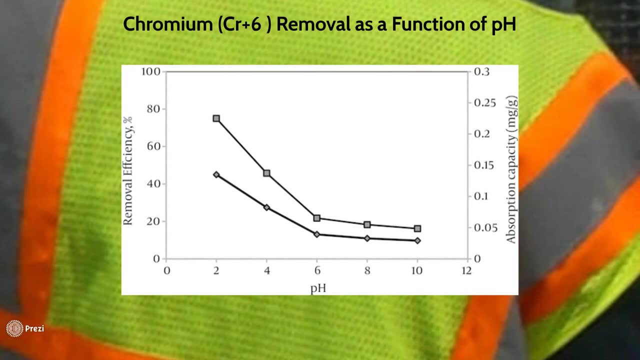 really have much of an impact in terms of decreasing the ability for it to sorb on to the ferrohydrite, and this next graph here is a similar one. again, I'll call your attention to the x-axis being pH from a zero to twelve. 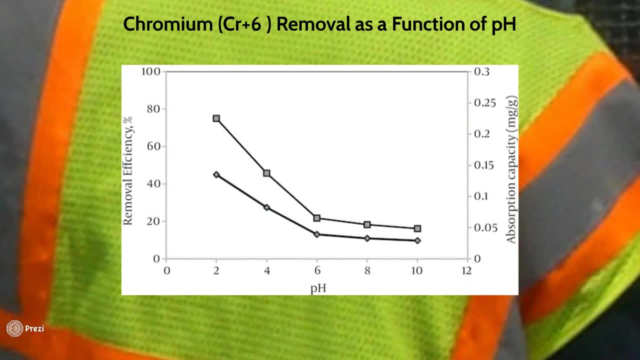 don't worry about the, the y-axis on the left, its removal efficiency. but to stay with the same terminology or units of expression from the prior chart, look at the y-axis on the right side for absorption capacity. if you're at the top of that at point three, it means in that pH environment these materials are. 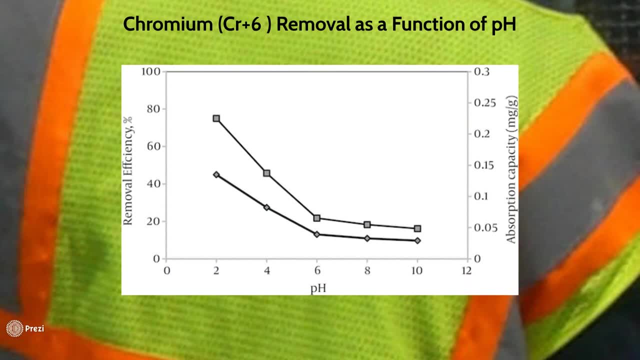 readily absorbed to other products or other compounds, meaning that pH is actually at the top of that pH. so you can see that the overall trend is to go in a downward trajectory, where both types of chromium here that are listed are showing. as you increase pH you are decreasing the ability or the absorption. 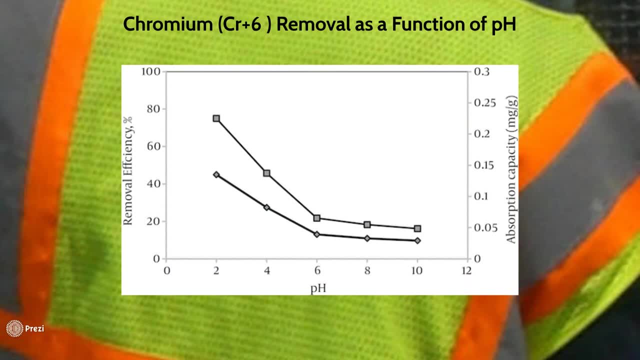 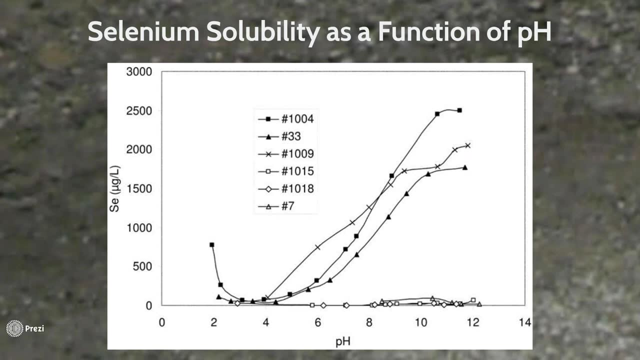 capacity, which means solubility is going to go up. and finally, selenium. you'll recall that there were four different valence states. this is actually showing six different selenium compounds. it's not clear on this graph here which of the valence states are represented by each figure, but that's not what's. 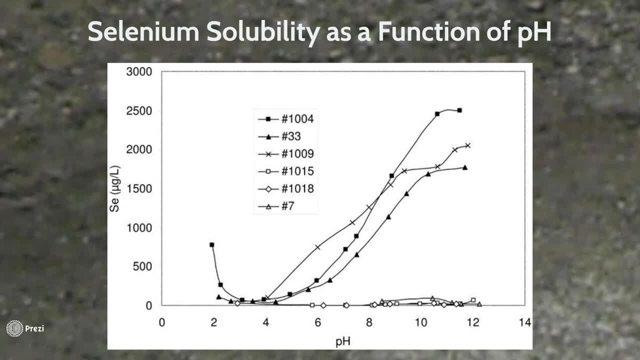 important here. what's important is there are two trends. with selenium again, pH along the x-axis, solubility expressed as micrograms per liter. if you multiply that by a thousand that would give you milligrams per liter. so we've got that unit because that's how the TCLP expresses its results. but the two trends I 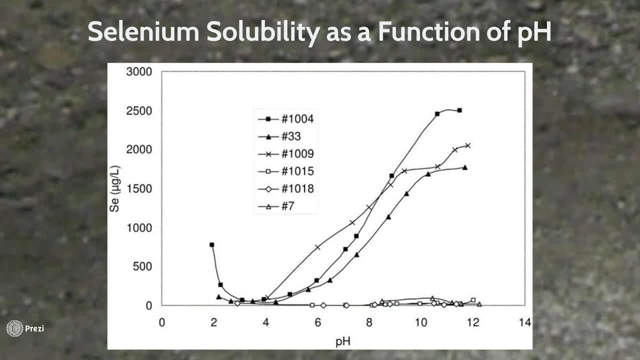 mentioned. if you move from left to right on the pH scale, you can see that for some selenium contaminated constituents that increasing the pH significantly increases the solubility of selenium. again, if we look at eight to eleven, lead and cadmium can be controlled by causing a hydroxide precipitant. 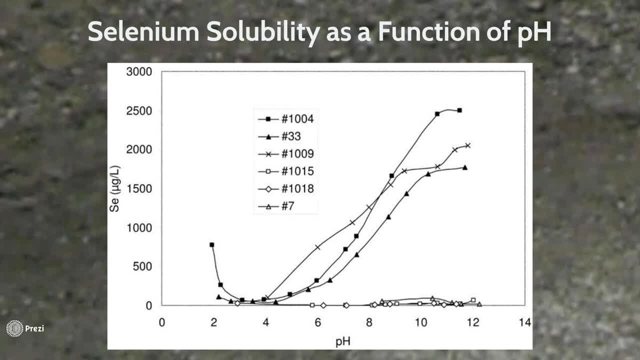 to fall out between a range of eight to eleven. here, if you have a range of eight to eleven, you're actually going to increase the mobility or the solubility of selenium. and then you can see for three other of the compounds, the, the individual shapes that are listed, kind of almost on the line between a pH of 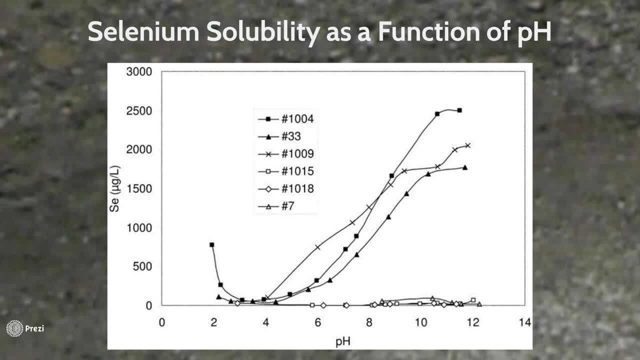 eight and twelve, you'll see that the solubility of selenium really didn't go up much, meaning that those forms of selenium weren't impacted by pH. so what I- what I hope I said in everyone's mind here- is you have lead and cadmium that can be controlled with pH chemical. 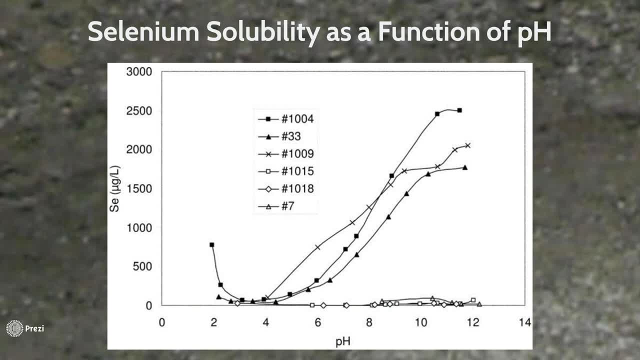 substitution, as well as encapsulation with arsenic, selenium and chromium. that's not necessarily the case and, as we've seen, increasing pH will actually cause these metals to increase in their solubility. so it becomes a real art to be able to come up with a solution that would work when you have both these. 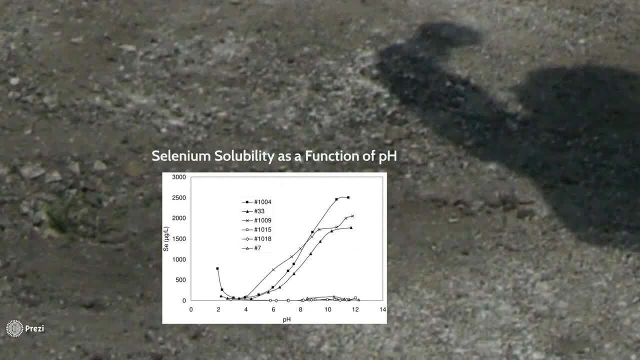 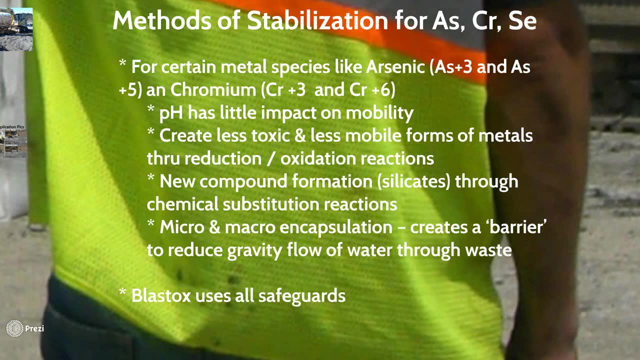 general types of heavy metals that would be present. we've talked about methods of stabilization for lead and cadmium and and review the the individual types of stabilization as we reviewed and alluded to. for chromium, pH has very little impact on on helping with the mobility and can evoke some 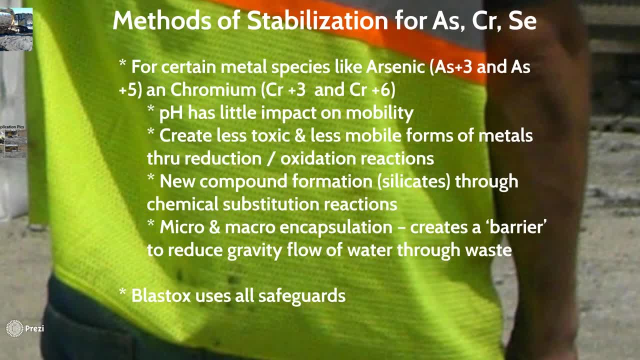 as we saw, actually increase the mobility. so pH adjustment as a standalone approach it is not typically effective with arsenic, chromium or selenium. what is effective is by taking that process or taking those heavy metals through a redox reaction or reduction oxidation reaction, changing the valence state of 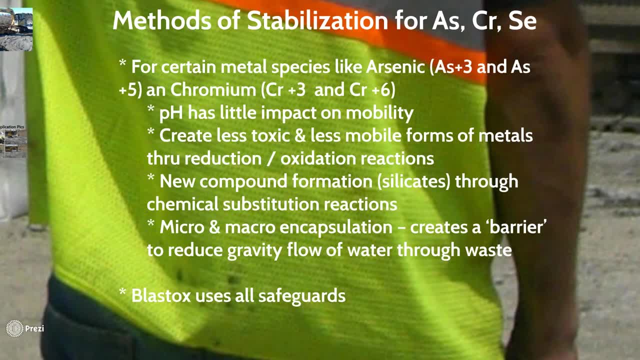 these materials to a point where they become less mobile by simply modifying the valence state and allowing them to be encapsulated by a silicate chemistry in in context of using our material, and if you're able to reduce the valence state to the point where it's not soluble, as is the case with trivalent 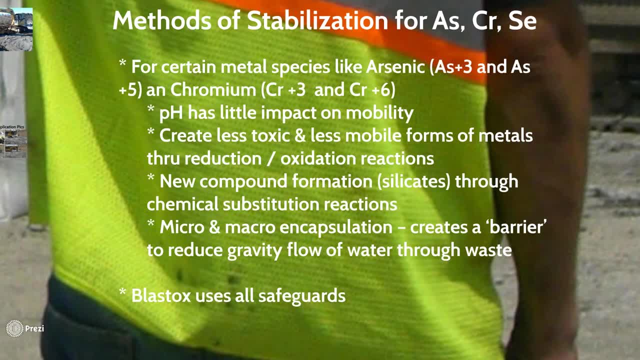 chromium, you would not need a chemical substitution reaction, because you've already helped to limit its mobility by simply changing its valence state, but by simply solidifying or encapsulating it. that would be the second required safeguard, in my opinion, to ensure that of these three types of unique and 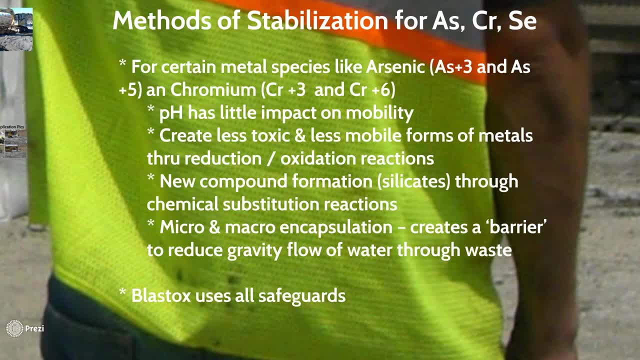 difficult to stabilize heavy metals, that you've got them suppressed so that they don't exceed the tclp test and just as a throw in there our blast docks by itself are, would stabilize the lead and the cadmium. and we have other enhancements, other redox of dry, granular or powder material that we create a customized blend that 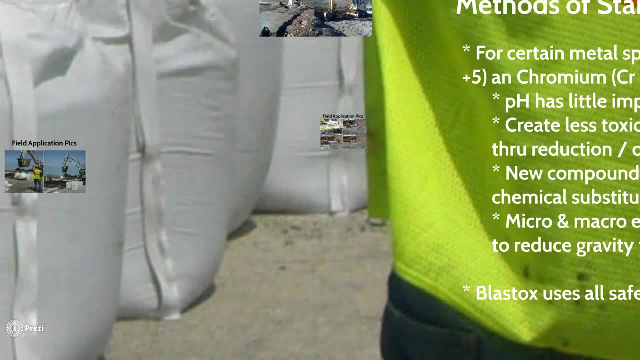 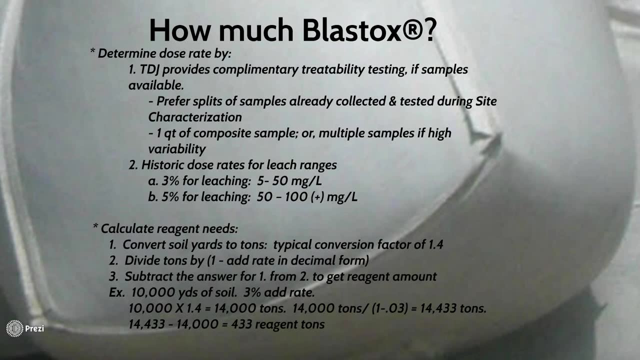 will achieve stabilization of these materials, and what I, what I wanted to do in this next slide is its title: how much blast docks? you can plug in whatever reagent name you went to there, but, but the same principles are going to apply. so how much reagent do I need to add? it's always ideal to get representative. 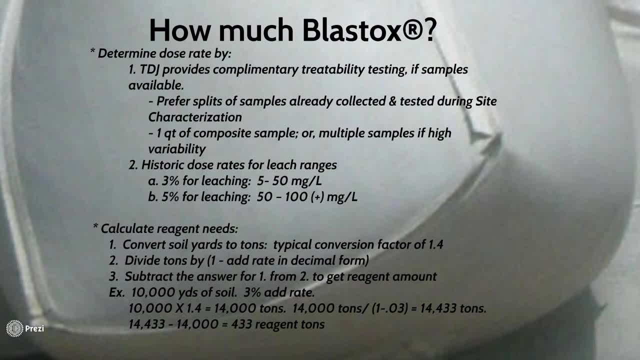 samples of a of a waste and do testing. we provide complimentary, that is, free treatability testing for people who are interested in using our chemistry. and, as we we lay out here, we prefer to get splits of samples that have already been collected and tested. that way we get not only a sample but we get the laboratory. 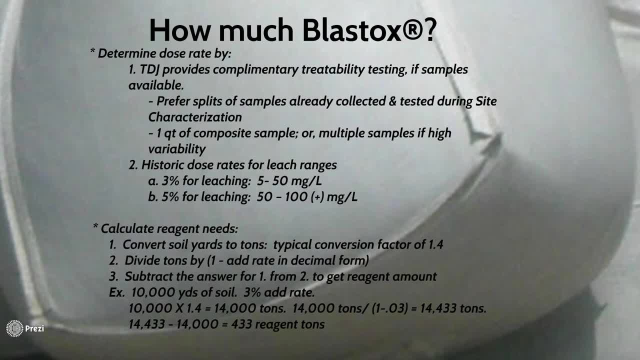 analyses to work this lightly. collection kau sextal, that test does give us knowledge about how premed remains actually, so that cising attenあぁ, I just wanted to give feedback to that question for the safety of chemistry, for that question. So that will help to inform which product and at what add rate we begin our treatability study. 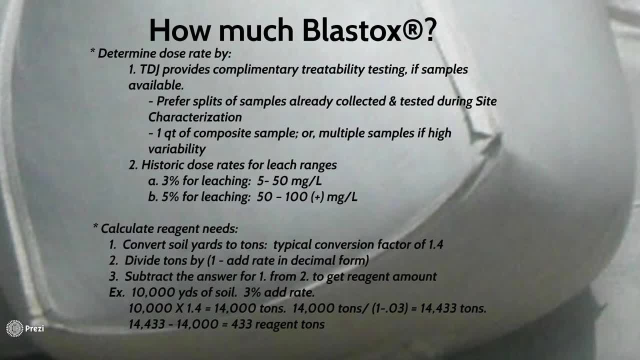 Again, it's important that we have a representative sample And if we have about a quart of a composite sample, if variability is uniform. there's probably some people chuckling right now about uniformity of variability. We've certainly seen in most projects you don't have uniformity. 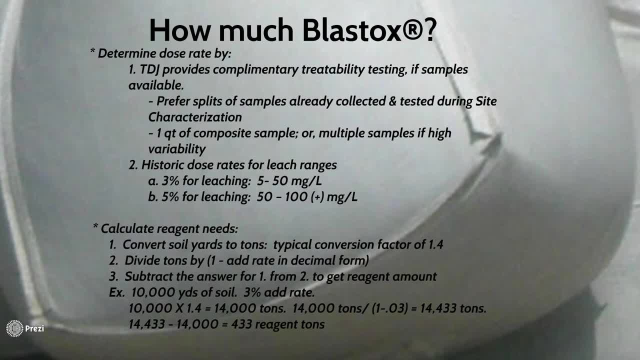 You do have a high degree or range of variability. In that case, we'd like to have a sample from each of the main areas of variability so that we can optimize how much you need to add, whereas you can either add a larger amount over the entire pile or, if you segregate it. 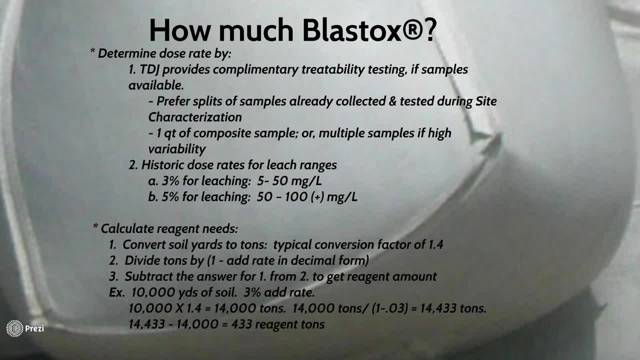 we can do, as an example, 5% in the higher range or 3% in the other range. If we don't have samples, we can still operate by knowing historically we have a history of experiences with our material, knowing that if it tends to leach between 5% and 50%. 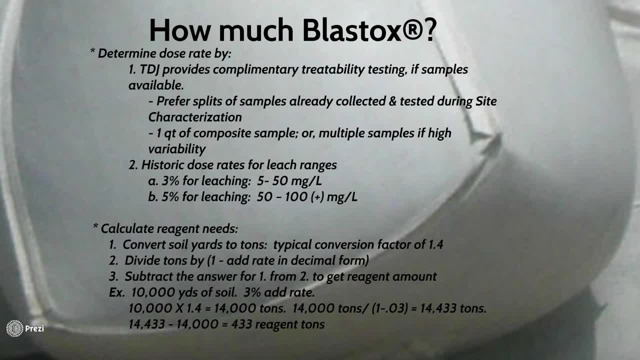 a 3% add rate will be effective, And if it's 50% to 100%. we've seen values that approached four digits there, meaning 1,000 milligrams per liter that we've been able to stabilize with a 5% add rate. 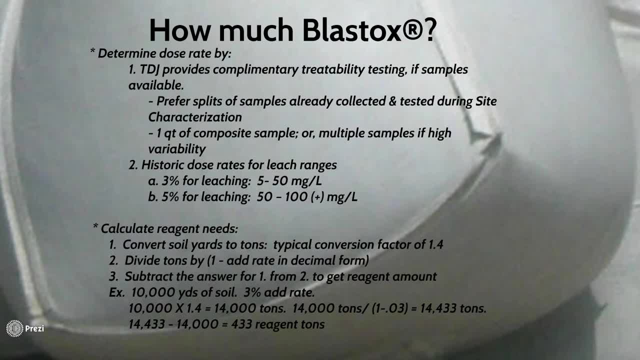 And these are typically add rates for lead and cadmium, As we'll see here in a little bit. when it comes to arsenic, selenium and chromium, it tends to require a slightly higher add rate. So either we've tested it or we've looked at the lab reports. 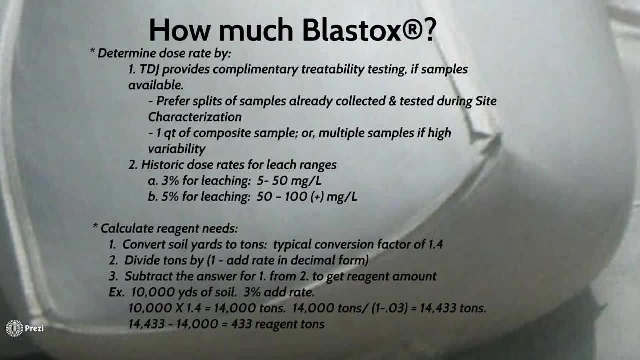 and we say we're going to use as an example a 3% add rate. And I know it's about 10.30 in the morning here in the middle part of America, maybe a little too early to do some math. 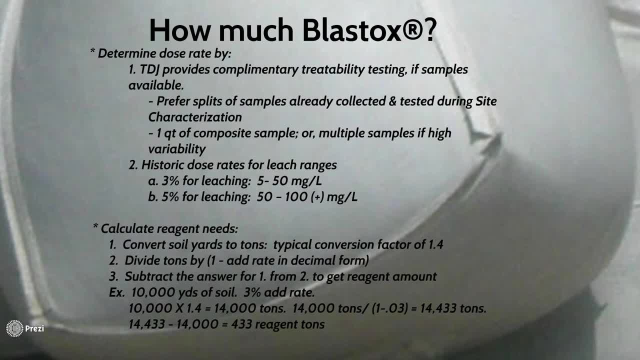 but this is very important because if we don't follow and calculate how much to add in this manner, we're going to come up with less material than is necessary, which might lead to a problem of improper or not uniform stabilization. So our example here is: we have 10,000 cubic yards of soil. 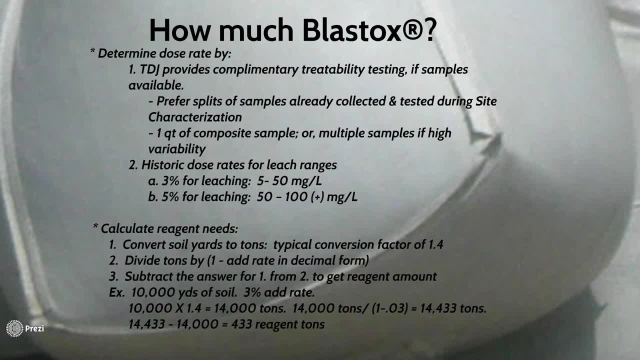 and we're just going to apply a conversion factor of 1.4 tons per cubic yard as a standard metric. And that would give us 14,000 cubic yards of soil, And we're just going to apply a conversion factor of 1.4 tons per cubic yard as a standard metric. 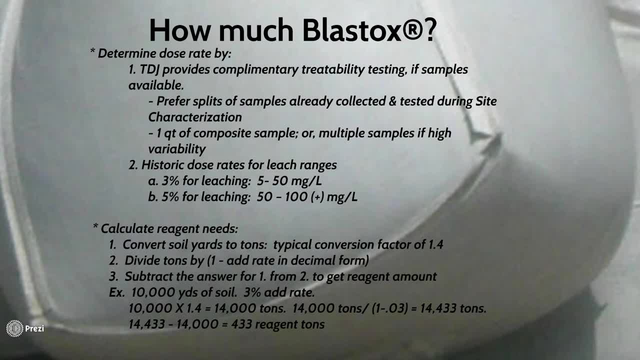 We sell our product on tons as a metric, not cubic yards, so that's the reason we calculate it that way. But in order to do it, you just don't take 14,000 tons and multiply it by 3%. If you did that, you get to 14,420 tons, which is less than what you would need. 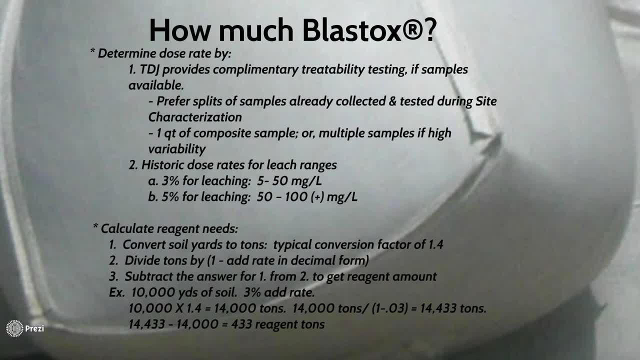 Here's the appropriate and accurate way to calculate how much I need to add on top of the 14,000 tons of soil. So you divide the tons, which is 14,000, by 1, minus the add rate, in decimal form. 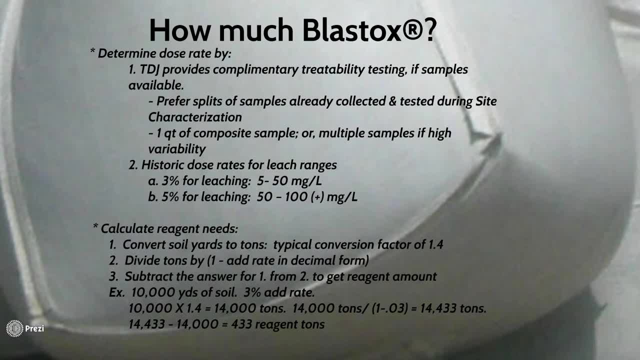 The add rate, as an example here, is 3% or 0.03.. So if you took 14,000 tons and divided it by 1 minus 0.03, which would be 0.97,, you're going to come up with 14,420. 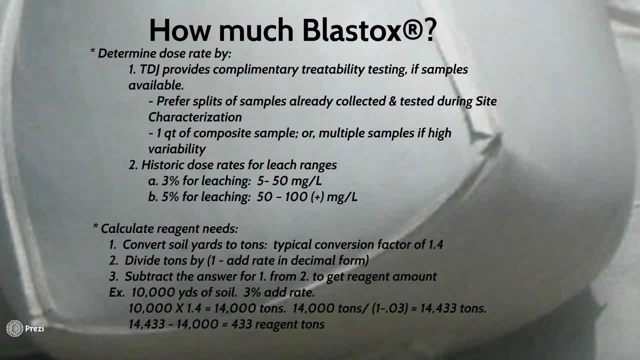 So that's 433 tons. The difference between that and what we started with, that is 14,000, is 433 reagent tons. Again, if you multiply 14,000 by 3%, just straight, kind of linearly calculate that. 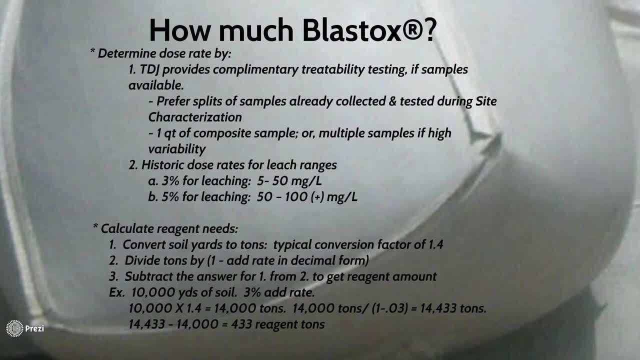 you're going to come up with 420 tons of reagent, which is 13 tons less than we would recommend, And as a result, we might be a little bit short on the dose rate overall. So hopefully that's pretty straightforward. If you have questions about that, again, I'd encourage you to submit a question to us on that. 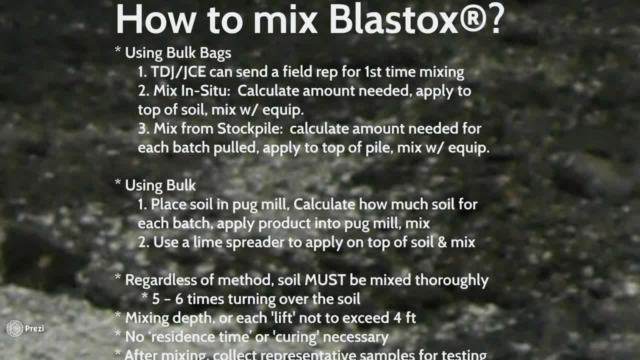 And now how to mix. So I'm going to go through and kind of again I'm saying how to mix blast docks. This would be appropriate with any other dry powder or granular material And using bulk bags, which is probably two-thirds to three-quarters of the projects we get involved in. 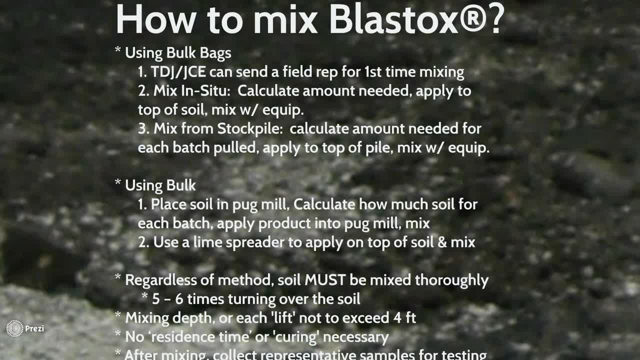 we'll certainly send a rep out if this is your first, And then we'll send a rep out if this is your first time mixing the material. And what we could do is, or an approach would be, if we've got, say, a 40-foot by 40-foot parcel of area. 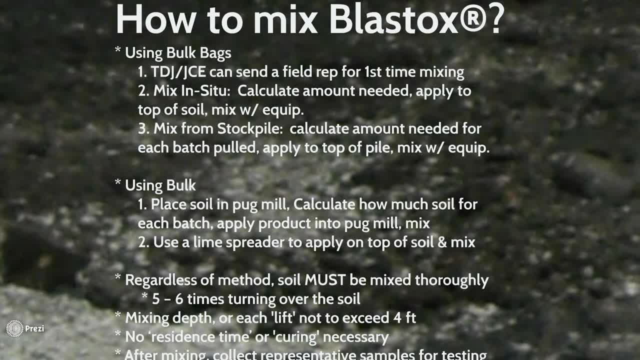 that's going to be contaminated down to about one foot. you'd calculate the cubic yards, Then you would calculate that to how many tons by multiplying it by 1.4. And then we go through the calculations that we did in the prior slide. 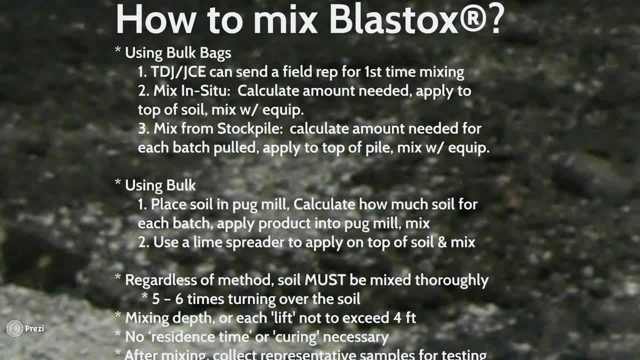 Whatever our recommended add rate was, we would calculate. We would calculate how much of our material you need to add on top of that 40-by-40 footprint, if you will, And then you simply with a backhoe or some other type of tool or piece of equipment. 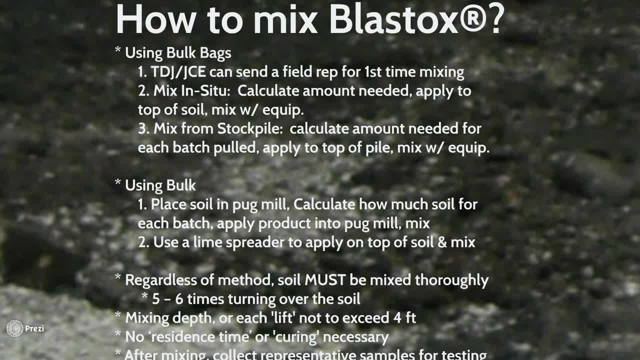 mix that material from top to bottom, ensuring that it's been thoroughly mixed, Whereas if you're using a backhoe, for instance with a bucket, you want to turn it five to six times. Now, that's one way of doing it. 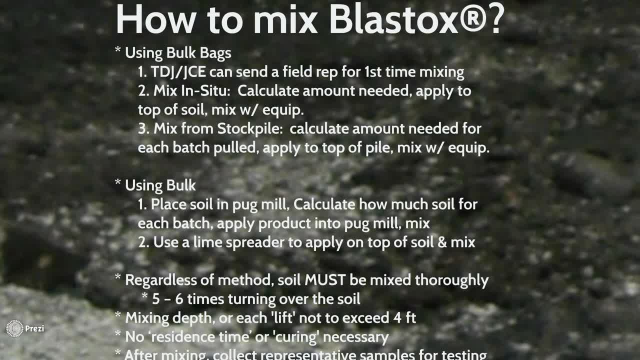 The other way of doing it is adding the material on top and then beginning your excavation where you're mixing the soil- Another type that's very common for very large projects. let's say you've got a 50,000-ton project and you want to work off of smaller piles, let's say 500 tons to 1,000 tons. 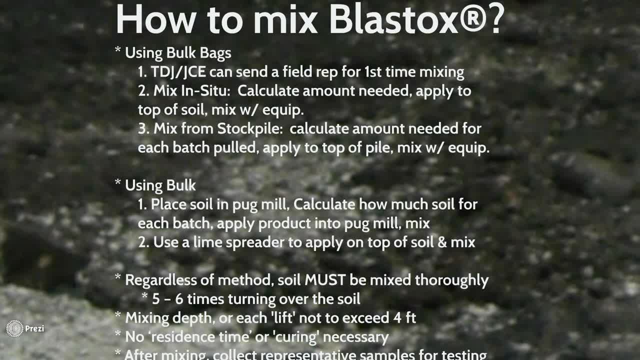 because it's easier to be able to mix 500 tons versus a pile that's 50,000 tons. So you'll segregate that 500-ton pile, Calculate again how much of our material you would need, Apply or disperse it to the top of the material and simply mix it again with either a backhoe or some other piece of equipment. 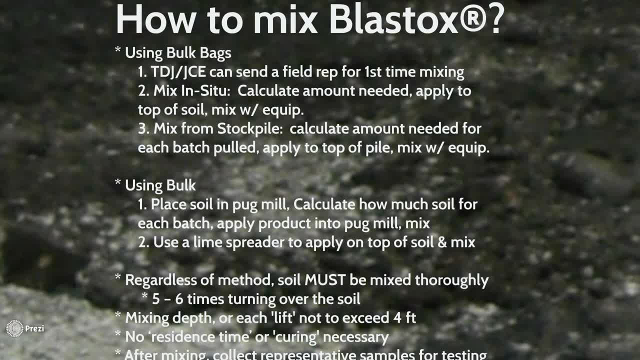 that would thoroughly homogenize the reagent and the soil to be stabilized. If you're using bulk, which again we can provide in bulk packaging as well, two different options that we've encountered in the field is one: you have a pug mill that's connected to a silo, and the silo will either blow pneumatically or gravitationally. 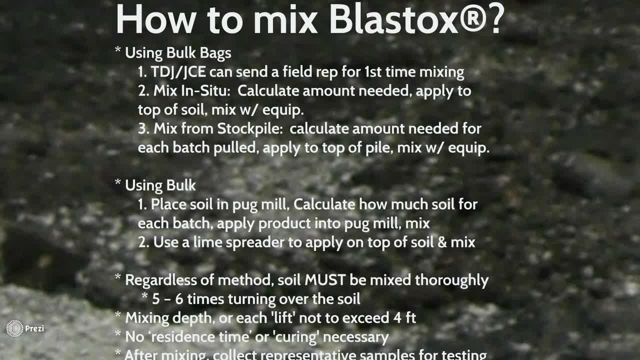 allow the reagent to flow into the pug mill, knowing that the pug mill capacity for soil is X, going through the calculation that we did before and determining the appropriate amount of reagent, adding that into the pug mill, activating or turning the pug mill on, and doing that for several revolutions. 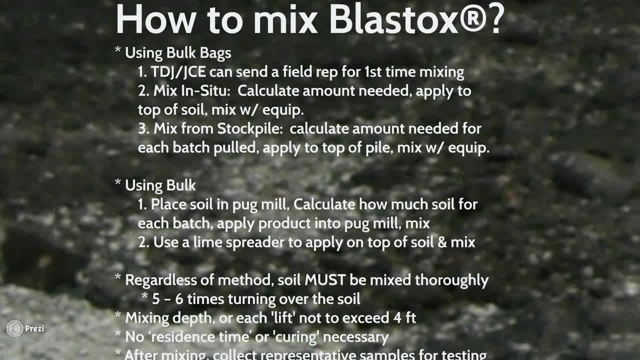 until you believe you've got a thoroughly homogenized soil. Another application for bulk are these trucks that are equipped with a tank that you can blow into from your on-site storage silo, and they've got either spray bars or a mechanism on the bottom that allows you to meter out a specific amount of material. 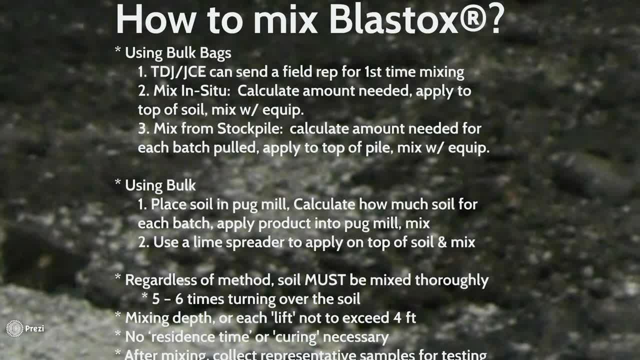 as you're driving over soil, And some of these units will mix it as it's being dropped out, or you'll need some kind of a large industrial tiller, if you will, to be able to mix it after you've applied it, with a line spreader or similar type setup. 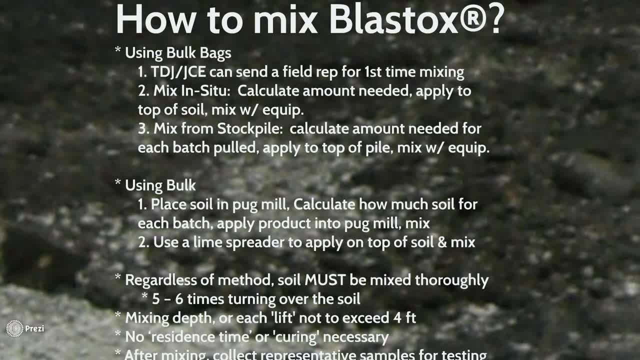 Regardless of the type of application, it's very important that you mix it five to six times, ensuring that the soil is thoroughly mixed, And if you're going to do this in lifts, we recommend not to do it in deeper lifts than four feet, because it's just simply too problematic to get it in there. 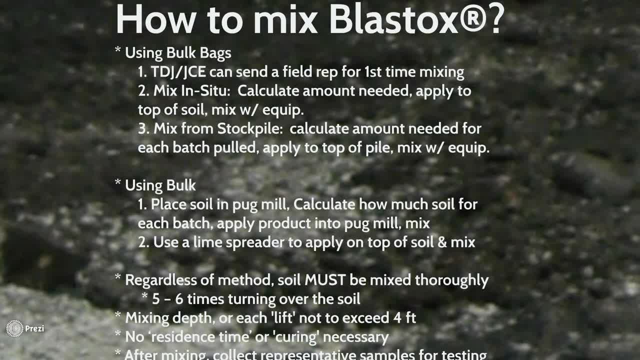 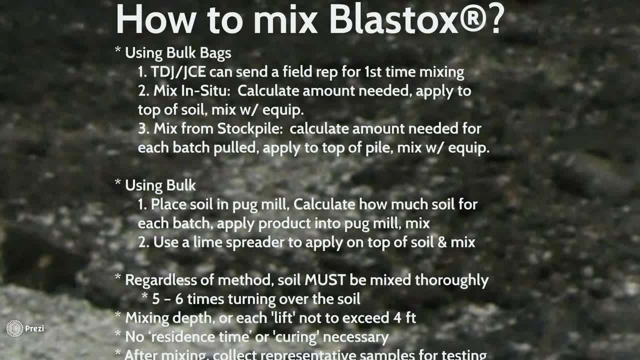 And to ensure that you've got good mixing going on With this material. it's different with other reagents, but there's no resonance time or curing necessary. you add it, you sample it. you still need to confirm that it came back non-hazardous. 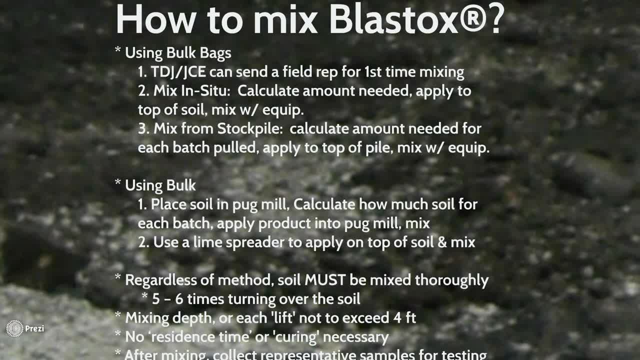 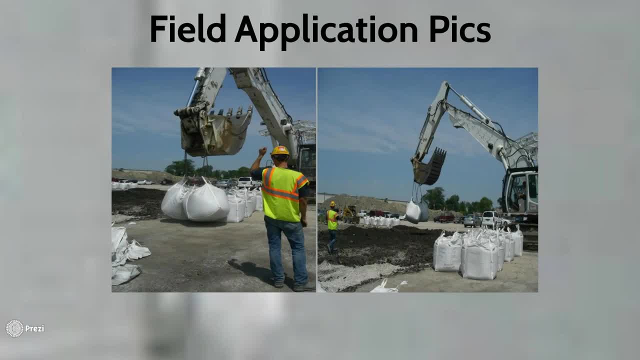 After it does come back non-hazardous, then you can send it off for testing. So I'm gonna go through a couple application picks here. Then I actually have a very short video of a different mixing head, if you will. that was placed on the end of a piece of heavy equipment. 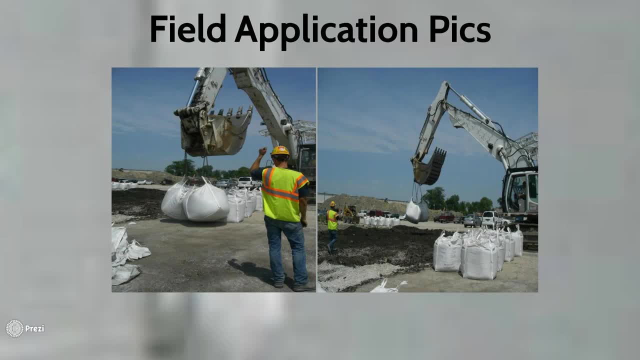 That's a pretty slick way of being able to homogenize the soil after the material has been added. Here are the standard bulk bags that our material comes packaged in. You can't see it very well in this picture, but at the very bottom of each bulk bag there's 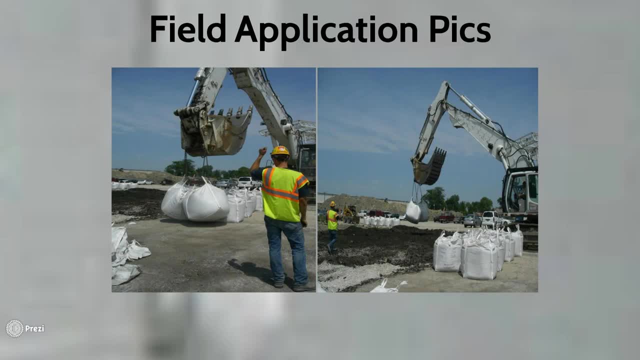 a spout with a choker or a regulator rope attached to it. You can open or close that and help to meter out how much material you want to drain out of the bag. As you can see, they've got a series of chains attached to the stirrups or the loops on the 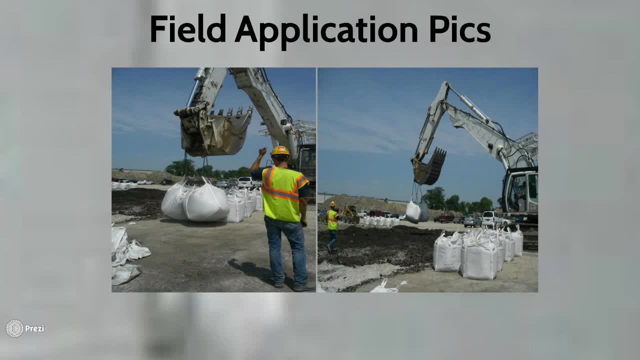 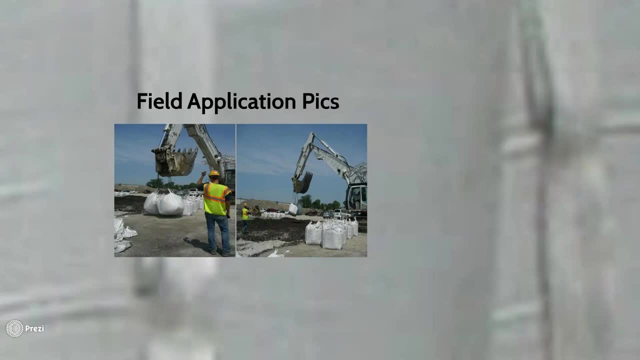 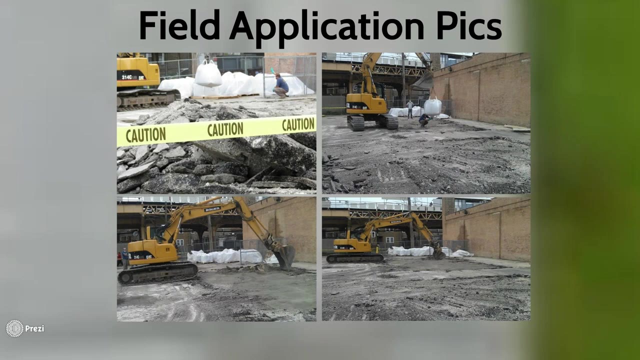 top of the bag. Then they can move that bulk bag around and simply dispersing it and applying this material on top of the soil, which would then be mixed at a later date, Later time, using a backhoe, not unlike the series of pictures here where, if you look, 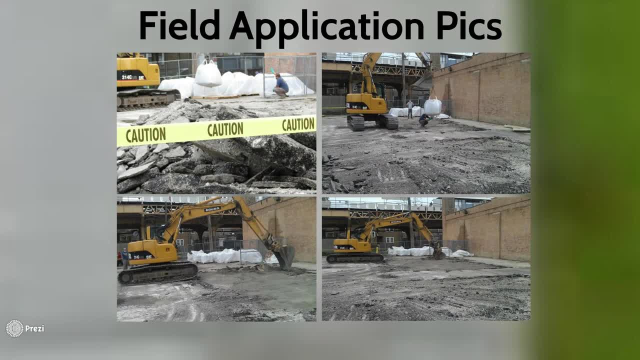 at the upper right picture, you'll see an individual just reaching underneath the bag to pull the spout out. And if you look at the lower left picture, they have already applied the reagent on top of it and now they're simply mixing it with the bucket on a backhole. 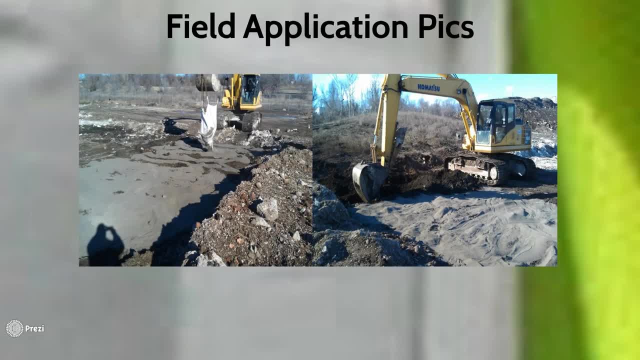 This is maybe a little big, better illustration were on the picture on the left you can see product literally pouring out of the bottom of that bulk bag and you can see they've been able to with with some good control, and a lot of these operators are really 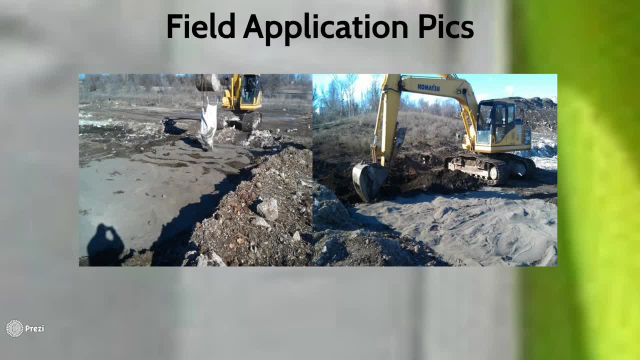 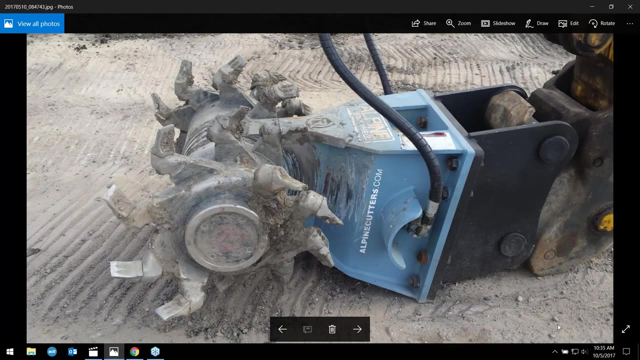 good at being able to kind of feather that material out and spreading it in a uniform layer. and then the picture on the right. you'll see where they're taking the bucket to mix it. now what I'd like to do is just quickly show you a picture of a different type of mixing head, and, as you can see here, it almost 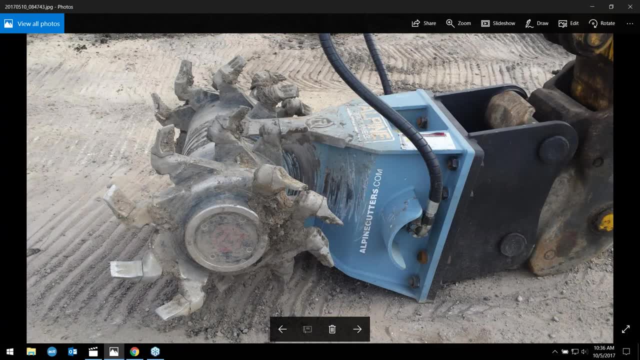 looks like some medieval barrel that's got all these spikes coming out. the video that I'm going to show you will show you these rotary arms in motion and how effective it is at mixing the waste along with the reagent. but the point here isn't to recommend one piece of equipment over another, it's just to 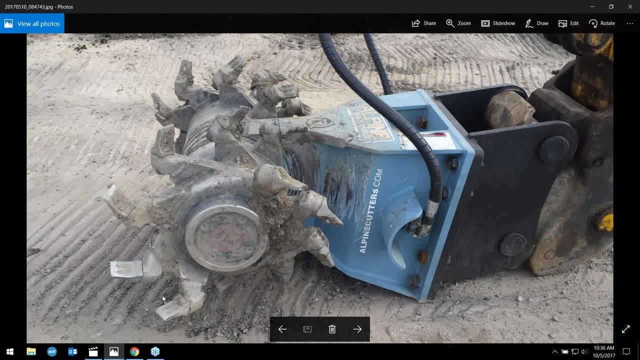 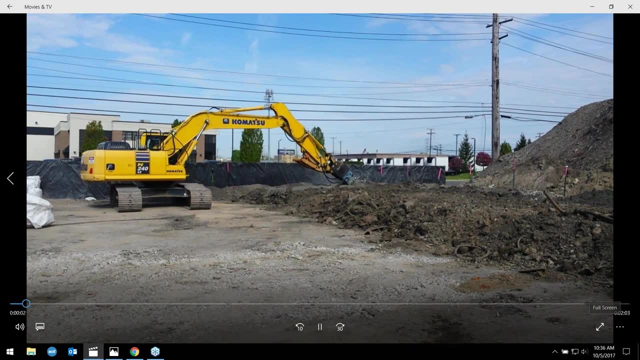 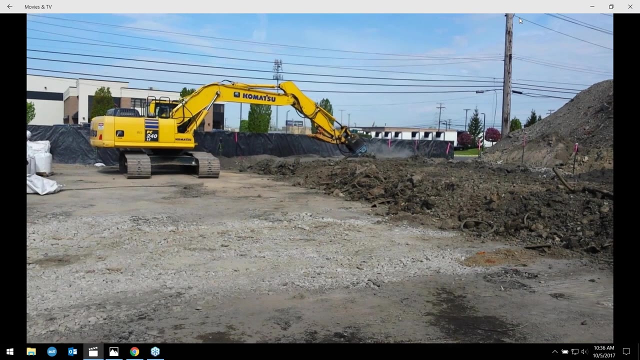 simply say some might be a little better than others, but there are multiple methods where you can mix the materials on site, so we'll get a little bit better close up here and I'm not going to make everyone endure a full two minutes, but as you can see that, 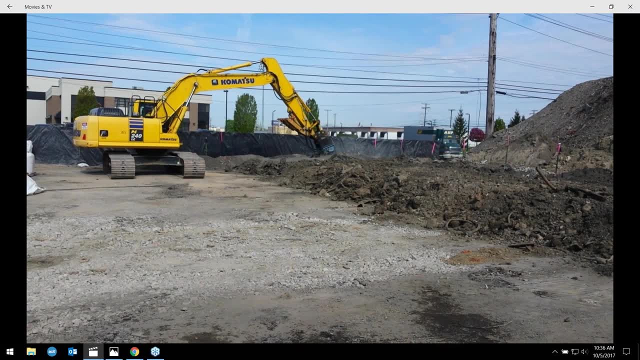 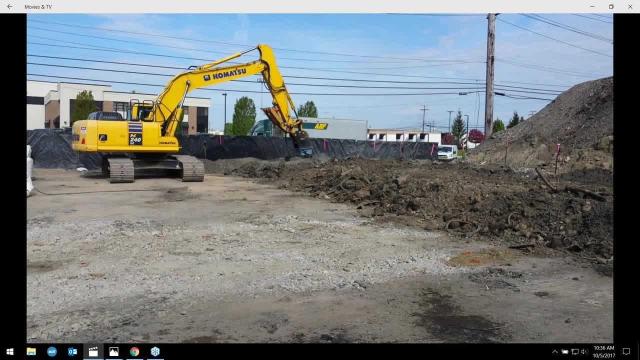 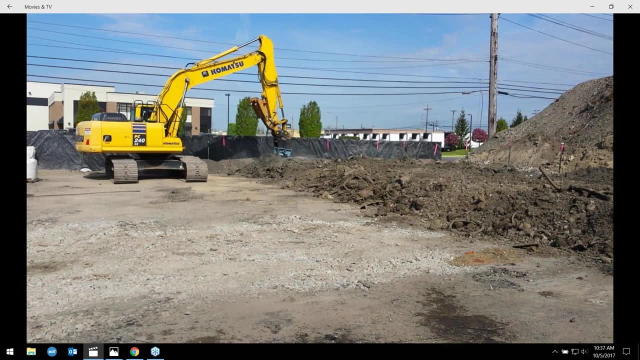 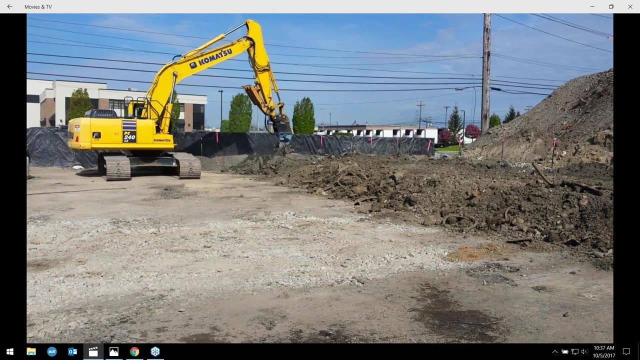 garden tiller, if you will, where it's mixing very thoroughly the soil as well as a reagent that they've already applied out of a bolt bag, and you can kind of see the bolt bag just to the left of that piece of heavy equipment there. I'll let this go for just another. 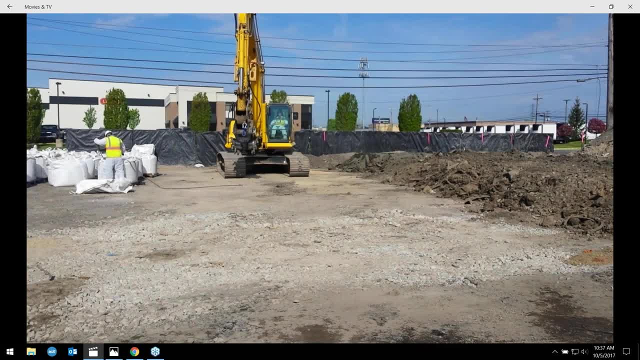 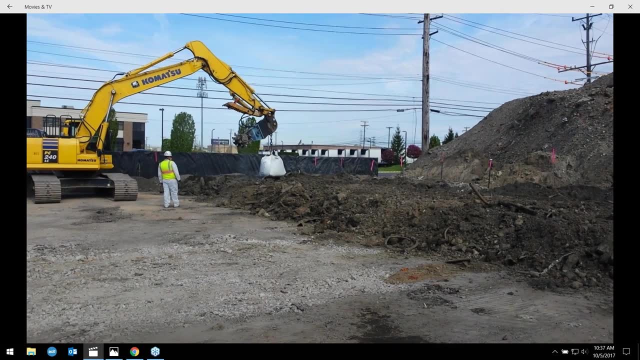 minute, but again you can see how easy it is for these operators to be able to mix from a, to be able to apply, I should say, from a piece of heavy equipment and either a spreader bar or a chain, and then, after spreading it again, this: this: 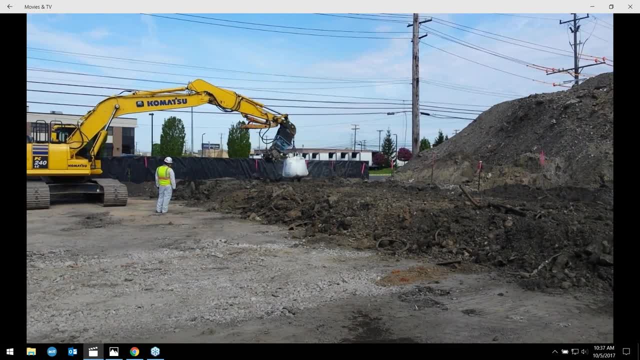 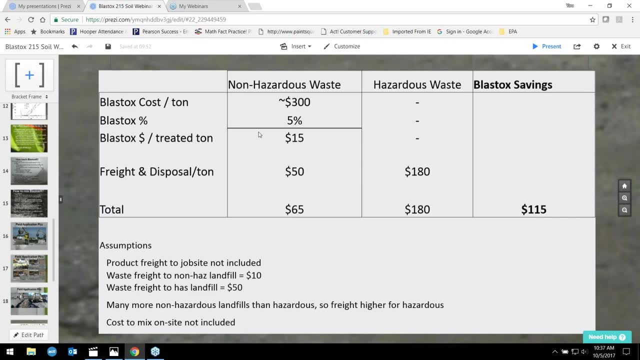 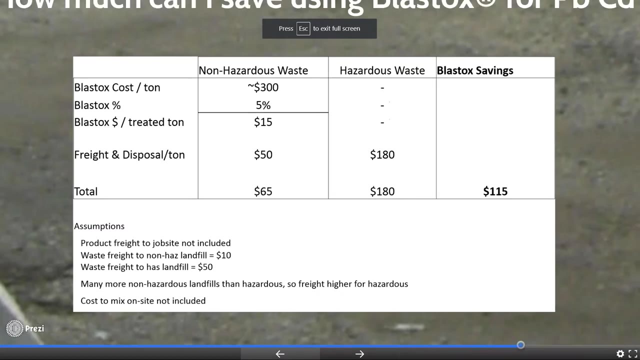 rotating head works quite well at being able to homogenize the materials. so I'm going to go ahead and jump back into the presentation here. we've just got a few more slides. if you can just bear with me, I just want to briefly talk about what. 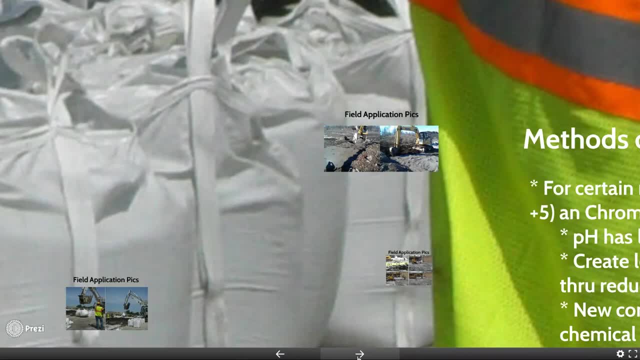 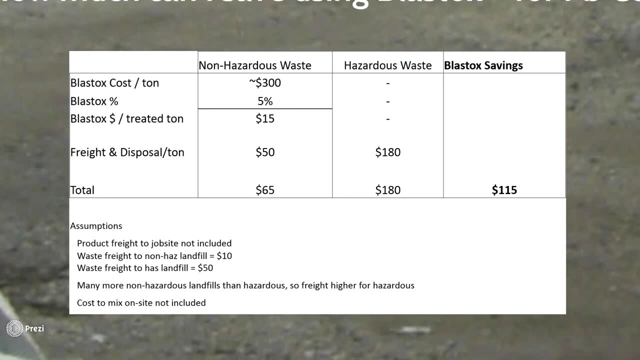 the what the cost would be, whether it's lead and cadmium, which is this first illustration, or arsenic, chromium and selenium, for the next one. the typical amount, a typical cost for our reagent is about three hundred dollars per ton and, as we alluded to, about a five percent add rate, if you just multiply that out. 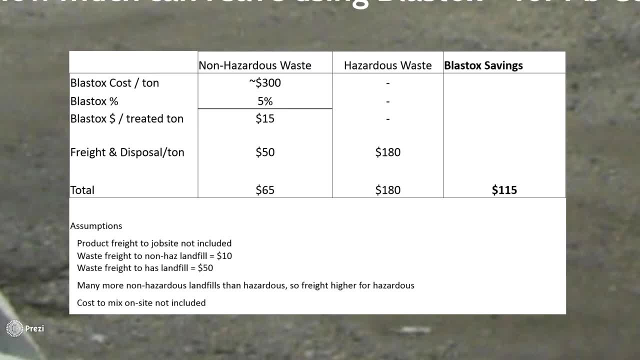 that works out to about a fifteen dollar per treated ton cost to treat the materials. on-site freight and disposal is about fifty dollars per ton on average for both for non-hazardous waste. so if you add fifty dollars per ton for disposal and fifteen dollars per ton to be able to stabilize, 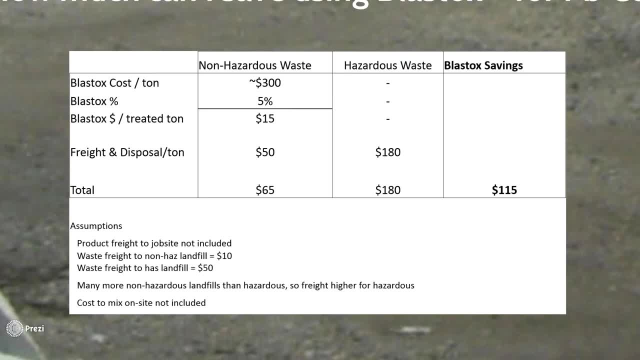 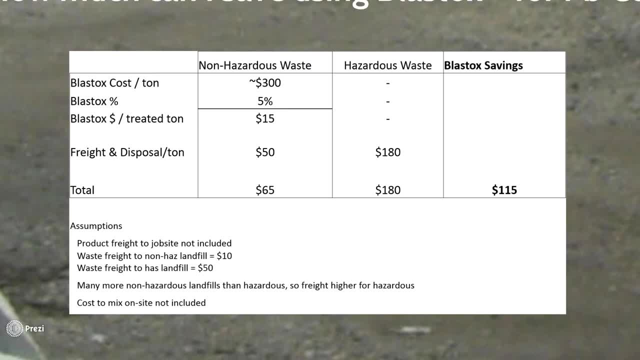 west here is about a hundred and eighty dollars per ton. I know as we get out to the coast those prices go up quite a bit, but in this application we're gonna save about a hundred and fifteen dollars per ton. so if you've got a project, that's. 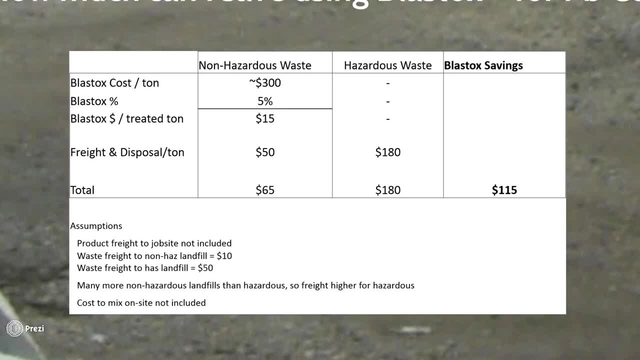 ten thousand tons, you can see quite quickly the use of this kind of a material would become very attractive. a couple of things that assumptions I do want to make people aware of is, as I said, freight to non-haz landfills about ten dollars. tip fees are about. 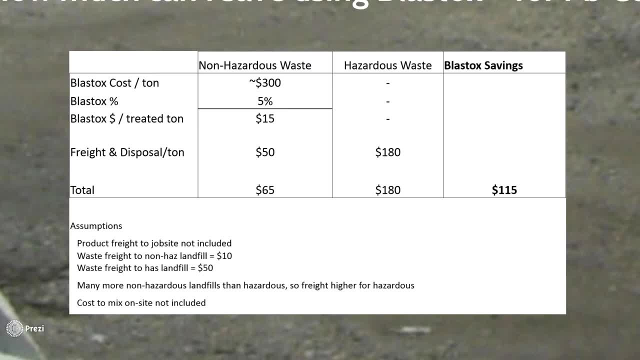 forty dollars, and I think that's a pretty accurate number. there are a lot more non-haz waste landfills than hazardous waste landfills, and that's the reason that freight is so cheap for non-haz waste, because the distance is shorter and they don't need the same type of certifications for hazardous. 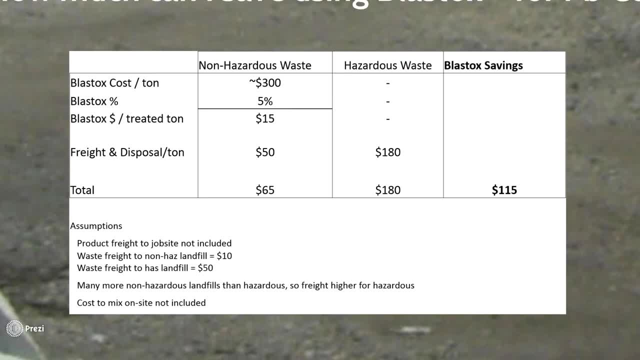 waste. you could transport those materials potentially hundreds of miles, which is going to make the cost of that tip fee and disposal package perhaps even higher than a hundred eighty dollars per time. also, what is not included is a cost of mixed blast ox on-site. what we tend to tell people is: 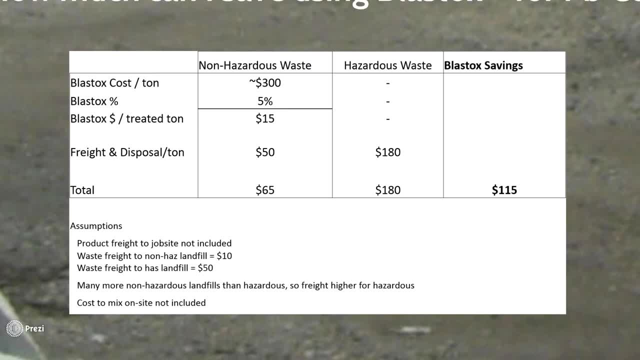 you're gonna know that better than what we are. but if you look, let's say, as an example, the cost of an operator and the heavy equipment was $300 per hour on an eight-hour day that's $2,400 if you were able to process a thousand tons a day. 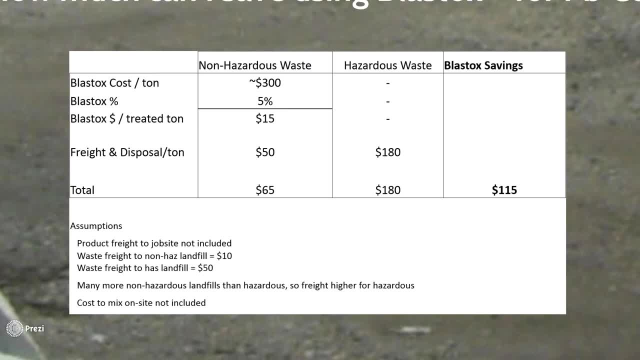 that's two dollars and forty cents per ton. if you could only do five hundred tons per day, that's four dollars and eighty cents, or about five dollars per ton to mix. so you can see the cost. to mix on-site doesn't really change the dynamics, or? 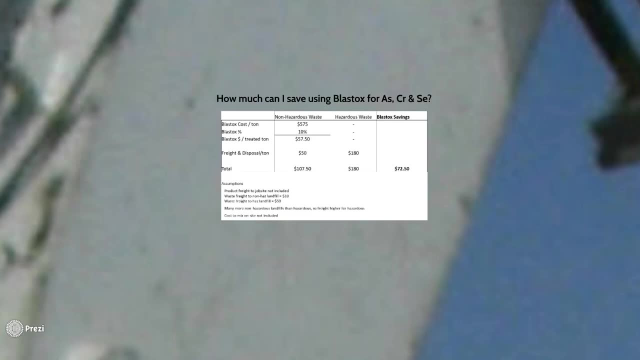 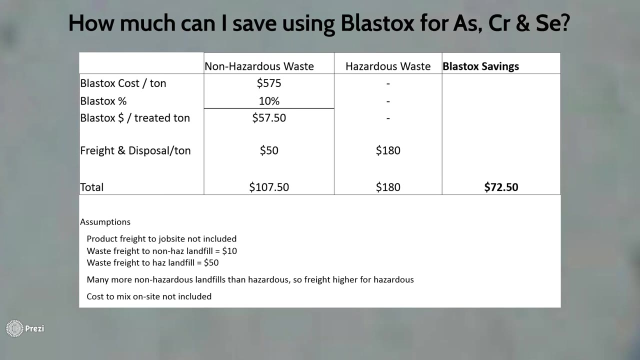 the cost savings that we're seeing here. as I mentioned earlier, arsenic, chromium, selenium do tend to require a redox material added to our basic chemistry, and that does increase the price of those materials. it's also been our experience that the ad rates tend to be around 10% rather than 5% for lead and cadmium. so 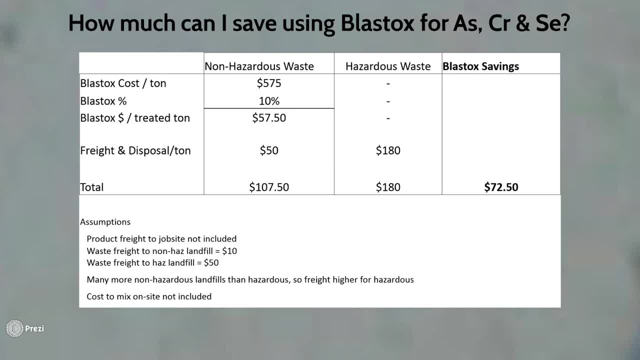 same assumptions here. same type of has waste disposal fee, which again I'm being conservative here because some of these more difficult to treat heavy metals. the landfill could charge you more based upon what their treatability studies suggest to them. but working through the numbers, it would cost about a hundred and seven dollars and fifty cents to apply the material on. 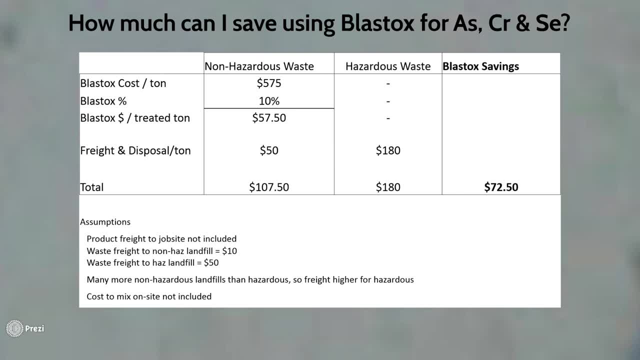 site and then to be able to dispose it off-site as non-hazardous waste, for a total of a hundred and seven dollars and fifty cents. same has waste disposal fee of a hundred and eighty dollars per ton for a blast dock, savings of seventy two dollars and fifty cents per ton. again, I have not added in the cost to mix it on. 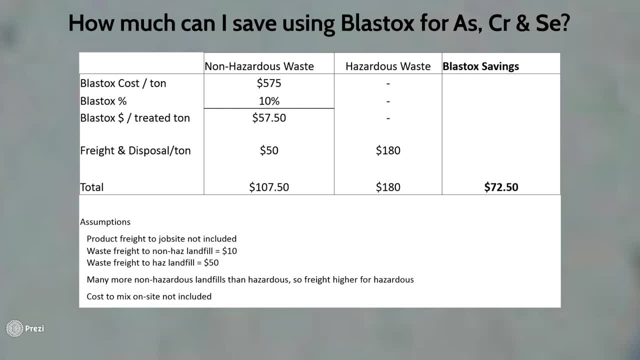 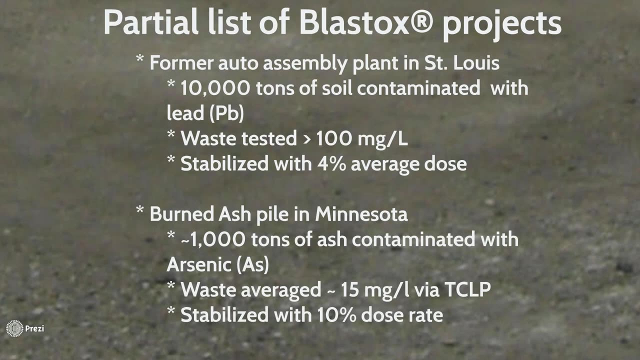 site you could plug in two, fifty or five dollars per ton or, if you've got a number you're more comfortable with, certainly plug that number into to to do your calculations there. I've just got a couple more slides left here where I'm just giving you a flavor for what we've. 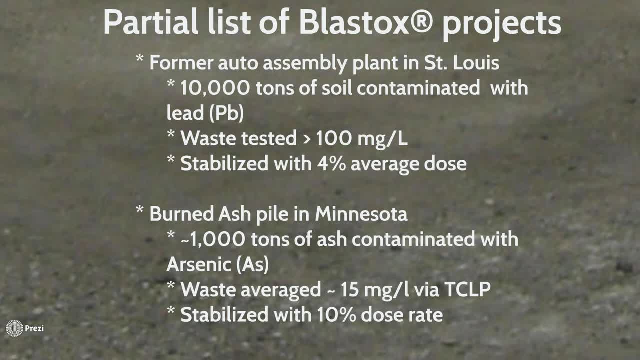 been able to see in terms of the contamination level and the average dose rate. this first one with a former auto assembly plant in st Louis where they had an e coat system, where they were able to apply the coating system in a way that required lead to be present well back in the day, before EPA was even in existence. they 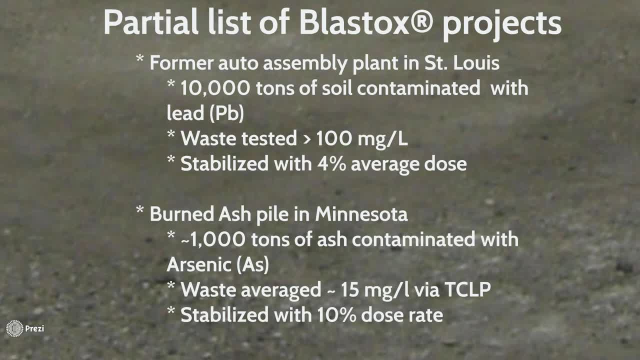 had a large burn area or burn trench where they would throw not only the eco waste but a little bit of everything else and burn it. well, that piece of property was purchased as they wanted to develop it, and what they were able to determine through testing was it had a 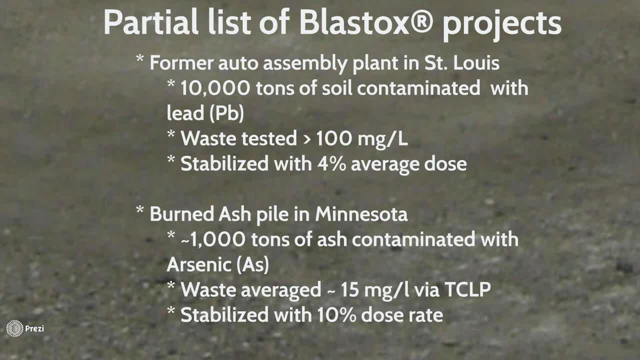 a average lead leachability of over a hundred milligrams per liter and we were able to to treat it at a four percent average dose rate. again it since it was lead. it was pretty straightforward. we've recently worked with a burned ash pile that was up in Minnesota and the burned ash contained pretty high levels of. 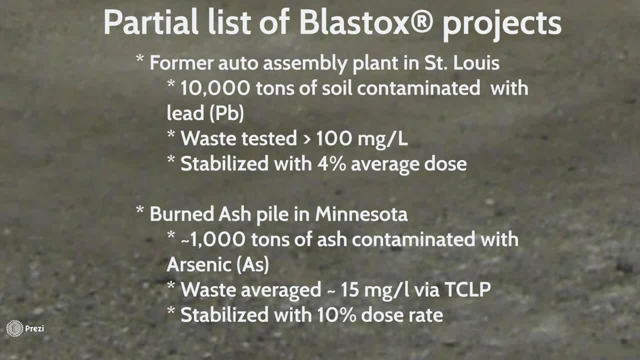 arsenic or it averaged about 15 milligrams per liter when tested via TCLP tests, and when we tested several samples with our blend of chemistries that have the redox reagent added to it, we were able to stabilize that for a 10%. 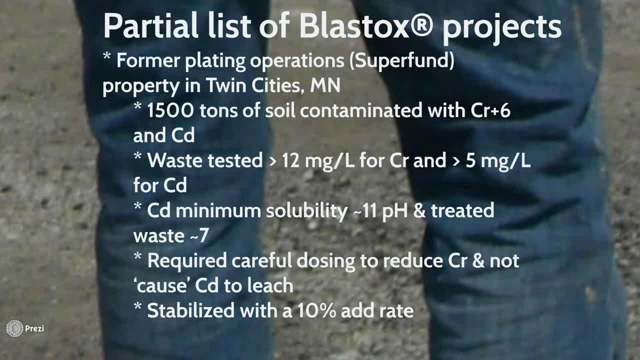 in dose rate. this next project was pretty unique in that it had both cadmium and hexavalent chromium. it was a former plating operation where it's very typical to see hexavalent chromium and that was a common contaminant for a lot of metal plating operations. that that 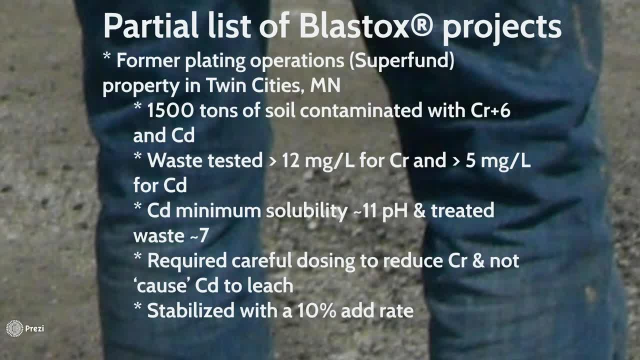 would have some environmental issues. this one happened to have both cadmium and chromium. I'll ask you to kind of go back in your recent memory here. cadmium had a minimum solubility range at a pH of 11 and chromium the data suggested. as you increase the pH value, you could actually either create more 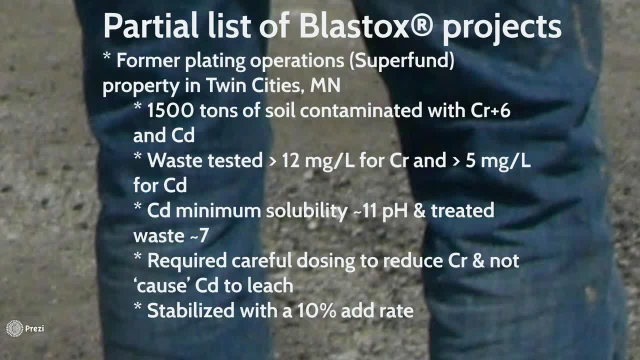 chrom-6 if there's chrom-3 that's present and or increase the solubility of chromium. so we had waste that exceeded chromium a standard of 5.0. the value here was 12. for cadmium, the TCLP limit is 1 milligram per liter and it was. 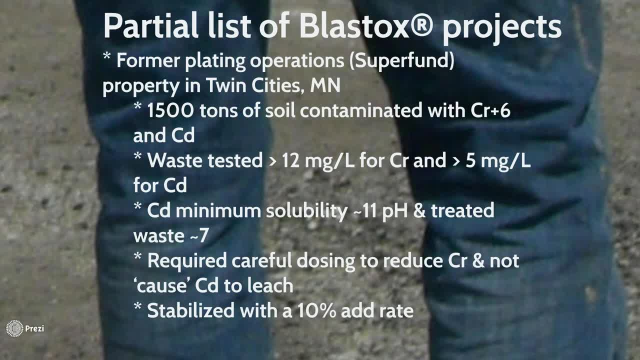 greater than 5 milligrams per liter. so we were able to come up with the solution that both minimized cadmium solubility, meaning that it was just pH adjusting. that's where the chemical substitution reaction came into play for the cadmium. for the chromium, we were able to reduce it to trivalent by 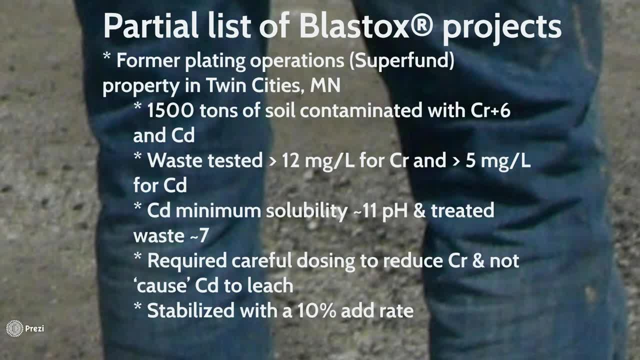 adding a material, a redox material, that effectively donated electrons to reduce it from hexavalent down to trivalent, and the waste finished at about a pH of 7, essentially implying that the cadmium was stabilized with chemical substitution because, again, if you relied upon its minimum solubility, 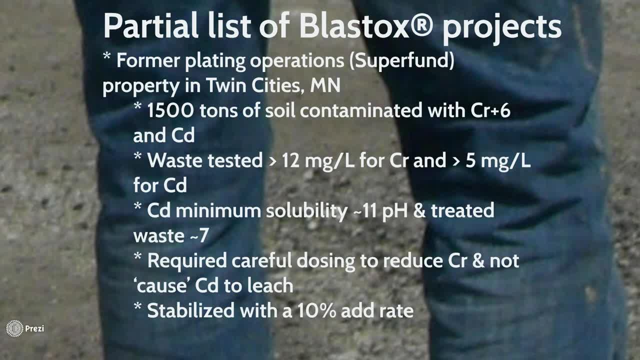 range at 11, which we didn't hit here. it couldn't have been a pH control mechanism at work here. so this, this material, this, this project, was very unique because we had to make sure we're stabilizing chromium without causing lead to leach, because our cadmium- excuse me, because a cadmium solubility at a pH of 7 would be. 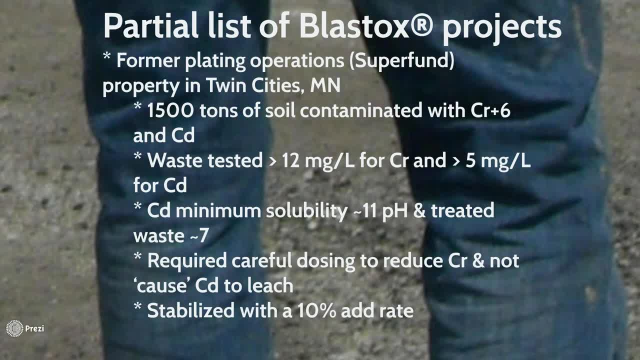 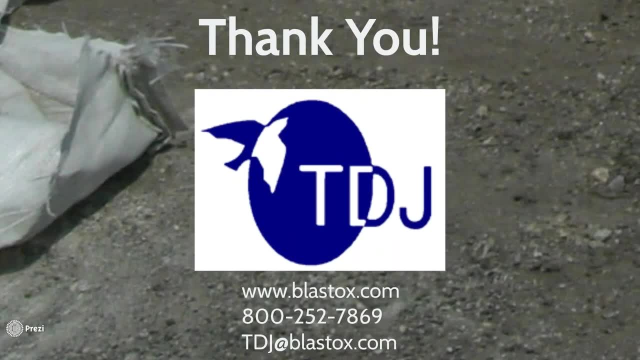 very, very high and I'm I'm happy to say we were also able to stabilize that material with a 10% add rate of the customized blend and at this point I'm going to thank everyone for participating in our webinar today. I'm going to bring up some 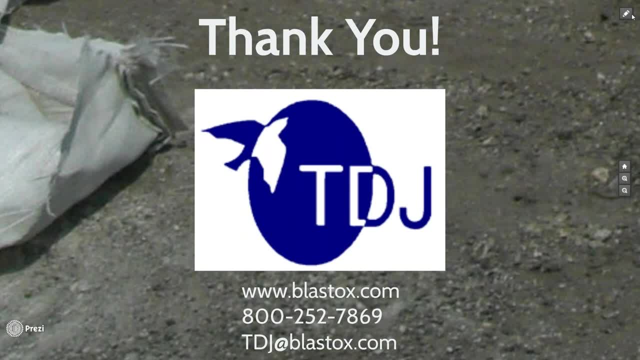 questions here. so if you guys can bear with me for just a moment, I'm going to read some questions out loud here. it looks like they were all public questions, so I do a really appreciate your submission of those questions. and the first question is: can this also work in a water treatment requirement? and Phil had asked. 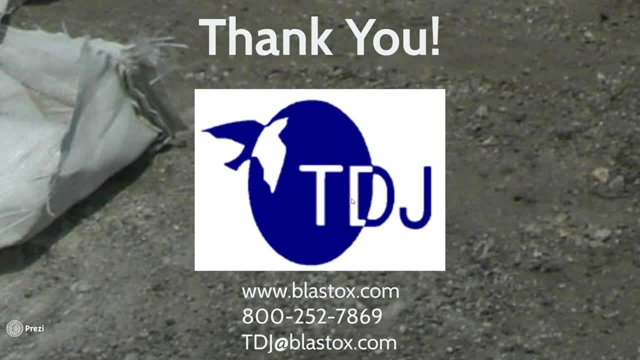 that question. so, Phil, thank you for submitting that question. very good question. it's one that were asked on a regular basis. our systems are designed to stabilize solid waste, not water waste. it's a really a completely different animal and, while there could be some beneficial use in water applications, our focus is really on solid waste. so to 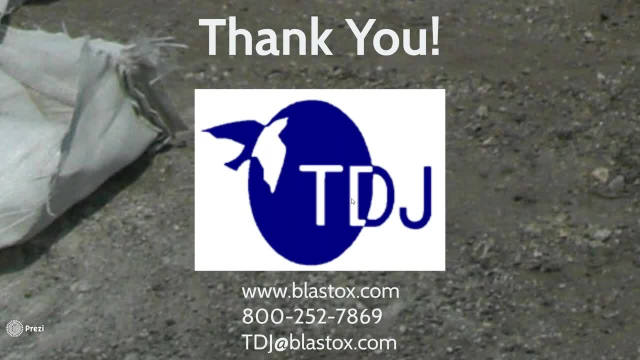 make a short answer, long, I guess, Phil. it's not really designed to work in a water-based environment. what are typical freight rates is another question that was asked, and I hate to sound like I'm going to evade that question, but the response would be well, that depends. 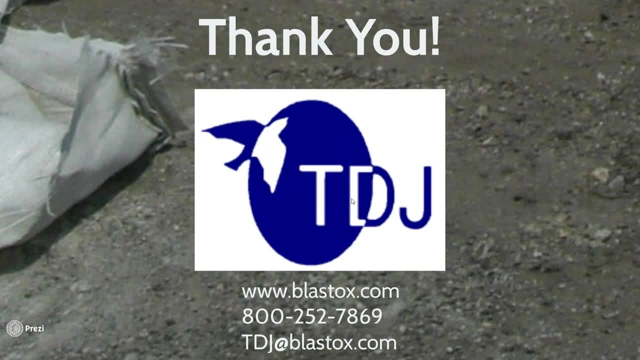 on the type of water that we're using. if you're on the west coast, we can transport the product in the middle part of the United States. if you're in in the middle part of America, in the Midwest, we can transport this product. again, that's where the product is produced, so I would say in the general Midwest for twenty to. thirty dollars per ton for the freight rate. if you're on the west coast and we can ship things intermodally, we can do that for about a hundred dollars per ton. so it depends on the type of the mode of transportation. if you can accept it intermodally would depend on is it pneumatic or is it in vans, because you're 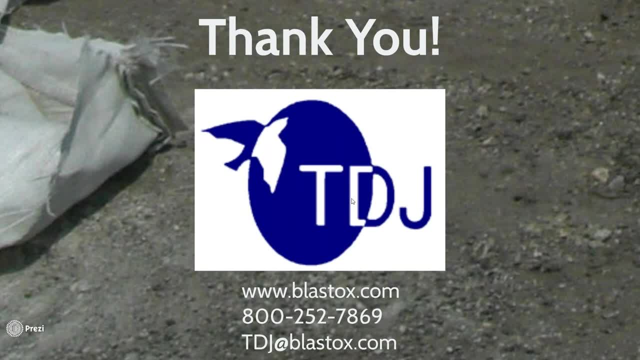 using bulk bags, and it would also depend on how far away from our shipping point in Peru, Illinois, that is located. if you have a specific project or just a general location that you want to share, we're happy to work with our distributor to be able to produce a freight rate quote for you. the next question was: 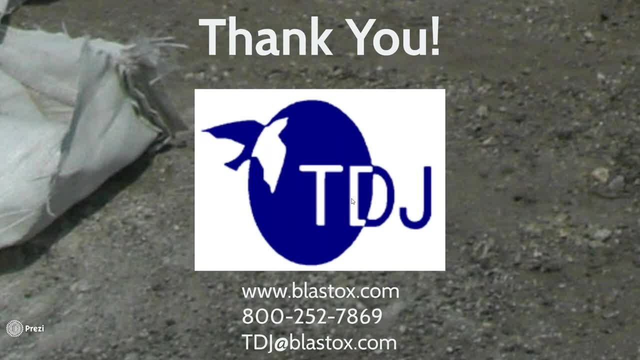 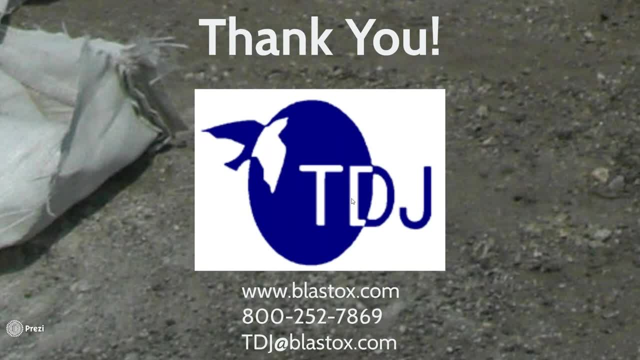 involved in a lot of testing and we haven't gotten involved with any projects that require that as a testing protocol. so, Todd, I think my question would be: I don't know, we've never tested it in those types of protocols, so perhaps that's some research that we 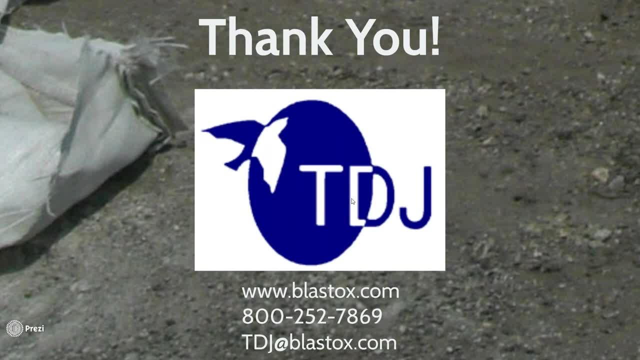 need to be conducting and we have. it looks like our last question that was submitted by Chuck Chuck, thank you very much for submitting the question. would it work to stabilize water treatment sludge? so that's that's kind of on the spectrum where we've got aqueous.